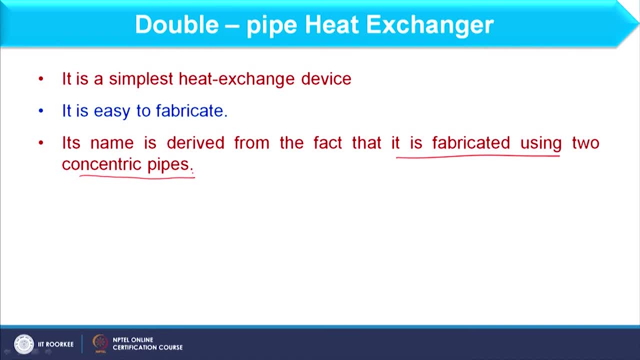 using two concentric pipe. okay, So therefore it is called as double pipe heat exchanger. One, fluid flows inside the inner pipe, while second, fluid flows in annular space between two pipes. okay, So that I think, functioning. you all understand very well, because when 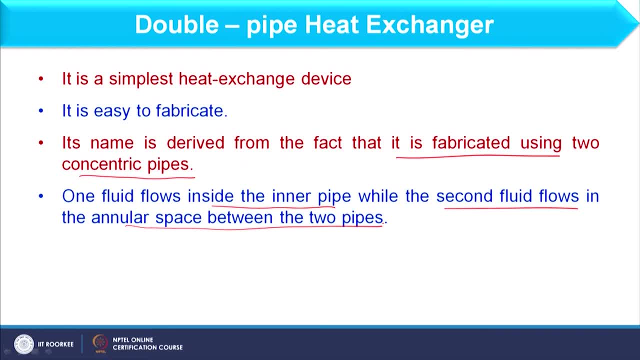 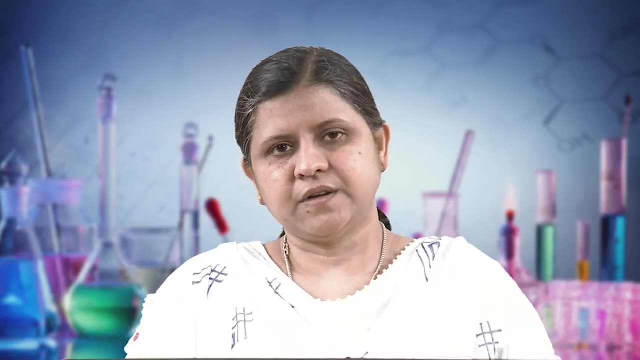 you do the research. you also have done experiments on double pipe heat exchangers, maybe in your second year chemical engineering course, So this heat exchanger is known to you very well, and it has other advantages, along with ease of fabrication and simplification. 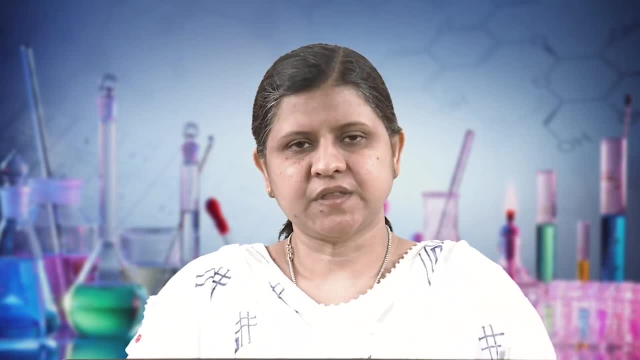 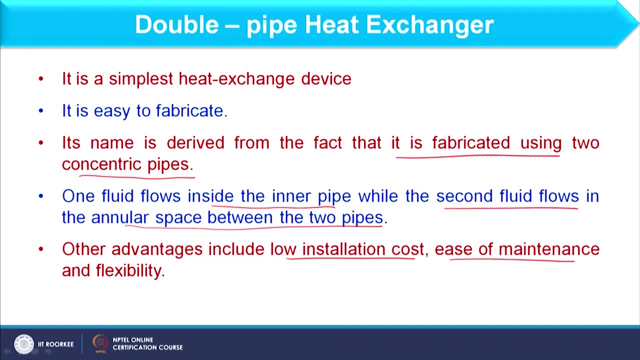 So let us get started. Page 1 of 11. Page 2 of 11. Page 4 of 12: design. The other advantages are: it has low installation cost, ease of maintenance and flexibility, because design is not much complicated, so you can consider ease of maintenance and flexibility. 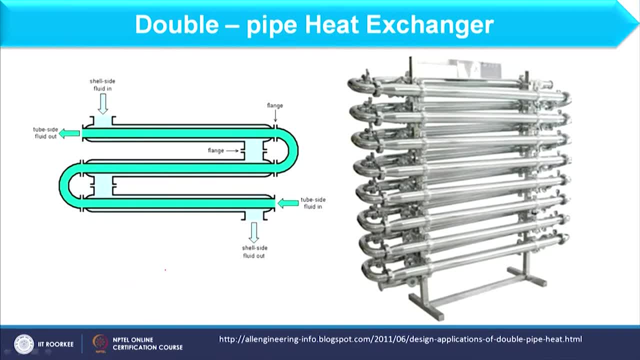 in such heat exchangers, okay. So here you see, we have this heat exchanger, double pipe heat exchanger. This is inner side and this is annular side. So one fluid is moving in annular side, okay, and then it transfers from here to here and 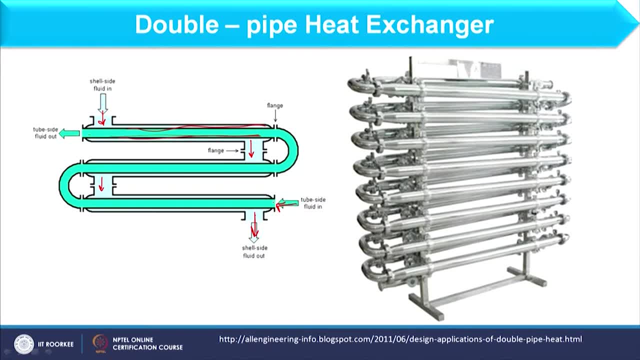 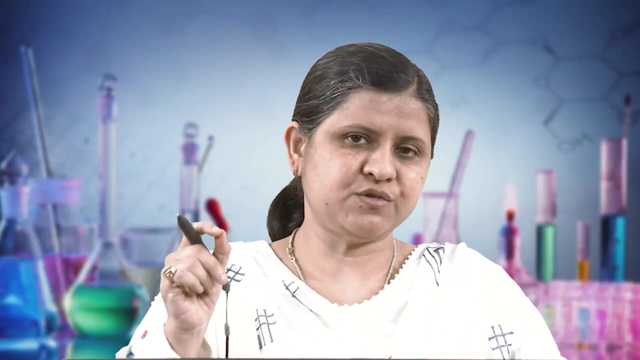 then exits from here, Another fluid is inside the tube and moves in serpentine manner. Now, if you consider this particular section of double pipe heat exchanger, this section is basically called as hairpin. okay, As usually we use hairpins. okay, it is this U shape. hairpins usually have U shape and 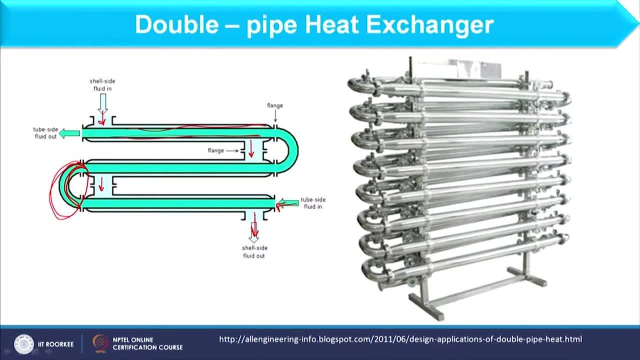 that shape is available over here also and therefore this section is called as hairpin. Now, if you see any commercial heat exchanger, it looks like this: okay, details are available on this side that you can go through. okay. So if you see, here I am having this commercial double pipe heat exchanger where we have hairpins. 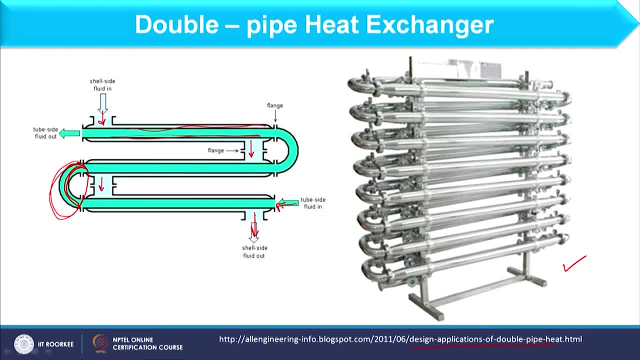 like 1,, 2,, 3,, 4,, 5,, 6,, 7,, 8,, 9,, 10,, 11,, 12,, 13,, 14,, 15, 16.. So if I consider both side, we have double pipe heat exchanger. 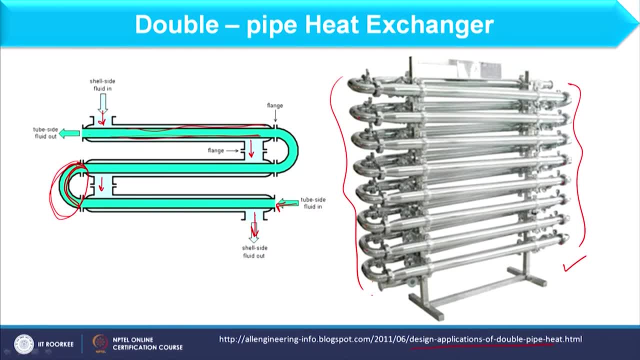 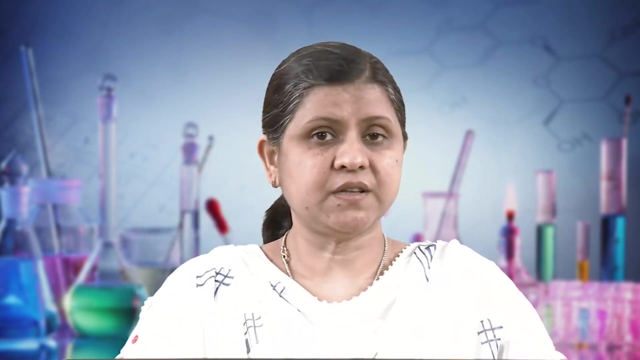 Okay, And inside this one fluid is moving and another fluid is in annular side, okay. So why I am putting this hairpin? okay? or why I am putting the U turn in double pipe heat exchanger? the reason is very simple: that it should occupy less space on the floor. 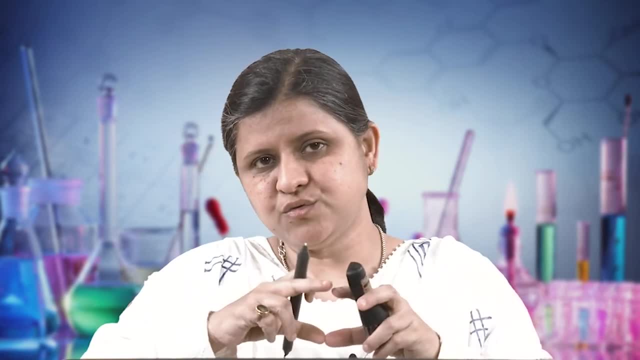 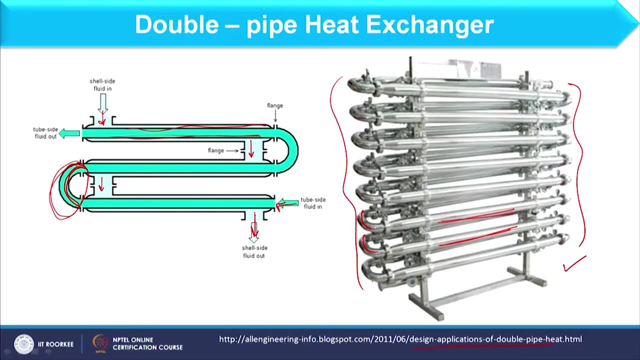 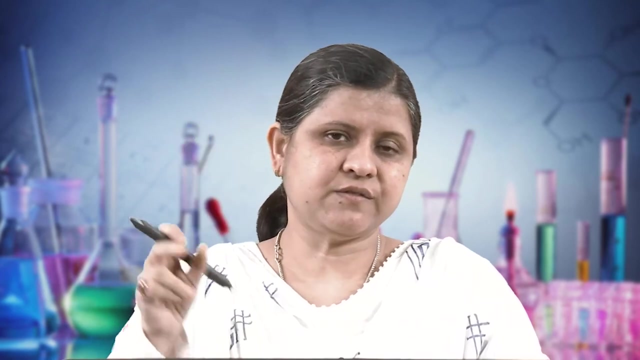 because double pipe heat exchanger- if you are considering the two concentric pipe right. So as we increase the area, the length of the pipe will increase significantly, okay, And therefore it will occupy more and more space on the floor. To reduce that, we can consider the same heat transfer area with less space while providing 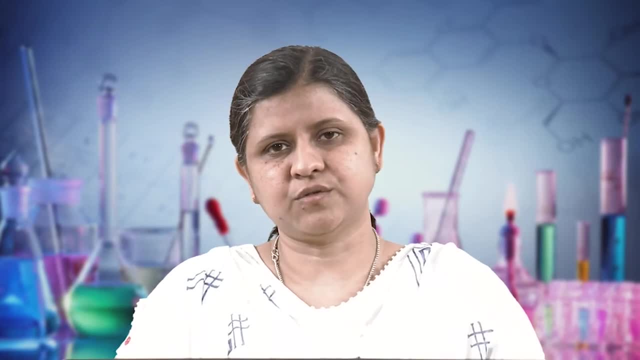 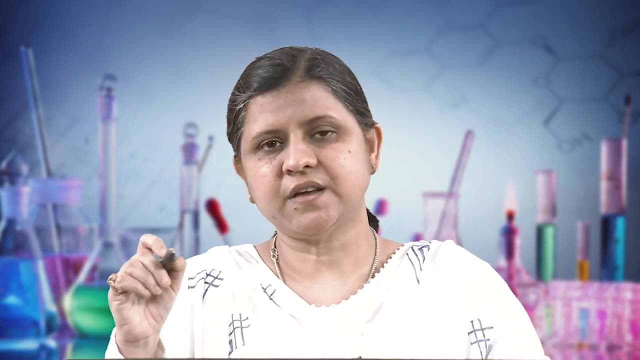 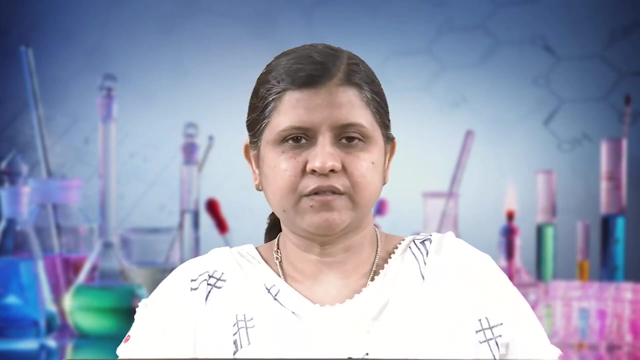 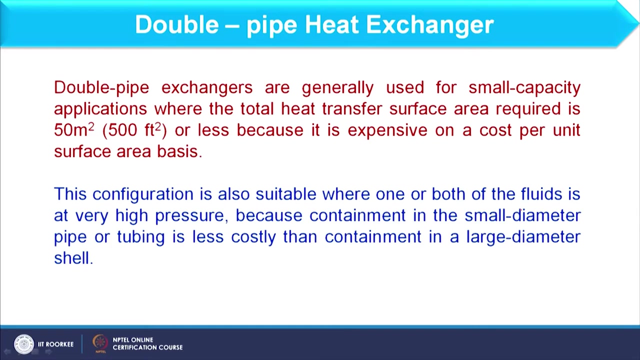 this hairpin type of structure, okay. So because of that, This hairpins and number of hairpins, along with the length, is very important criteria while designing double pipe heat exchanger. That point we will discuss when we will consider its designing. And here we are discussing some more important facts about the double pipe heat exchanger. 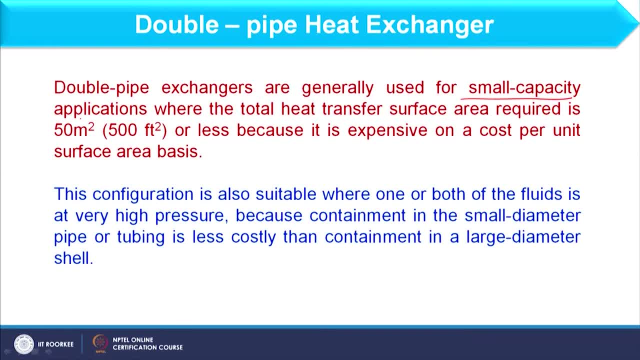 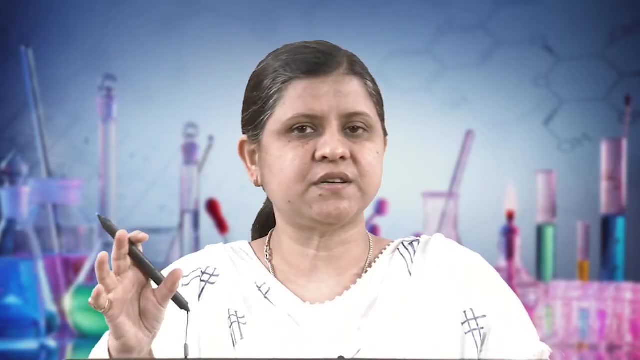 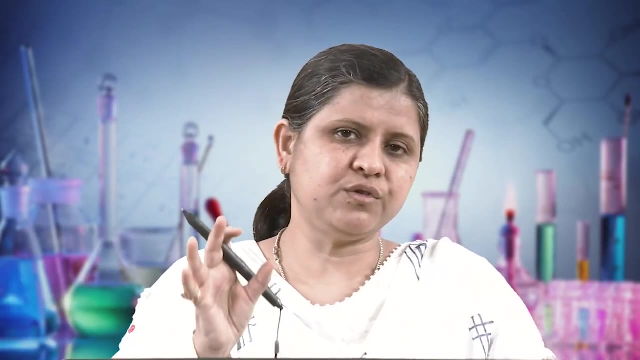 Double pipe heat exchangers are generally used for small capacity applications where heat transfer surface area is around 50 meter square or less than that. okay, Because though we are considering hairpin, but still it will consider sufficiently large area on the floor in comparison to other heat exchangers and therefore we do not use double. 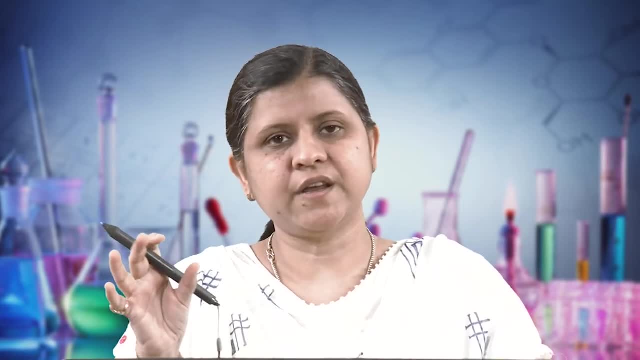 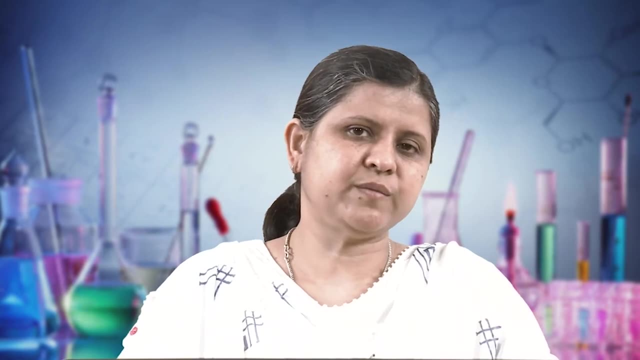 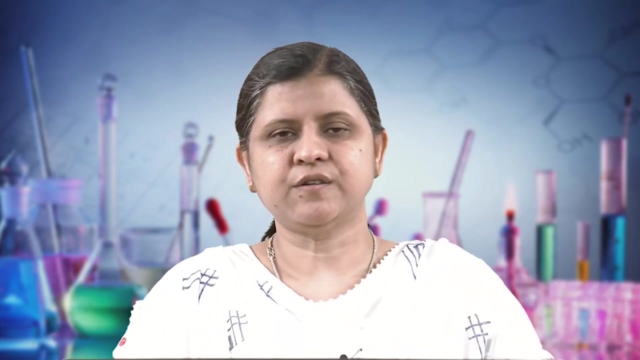 pipe heat exchanger for large load or for very high load. okay, Load, you understand the heat duty. okay, So heat transfer area up to 50 meter square, We can consider that. So double pipe heat exchanger and if I am finding more heat transfer area than that, 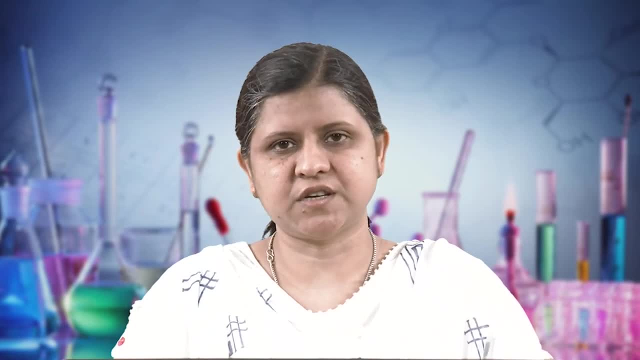 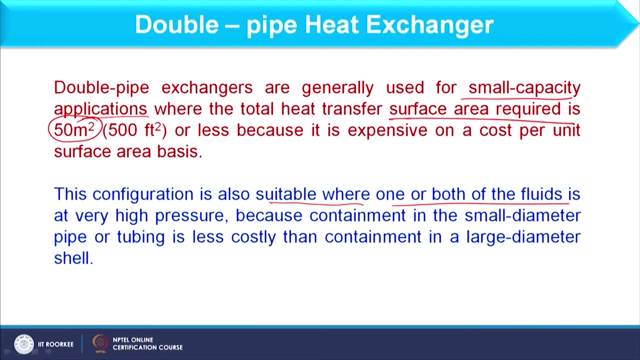 we should choose other heat exchangers, like shell and tube heat exchanger, etc. And this configuration is also suitable where one or more or both of the fluid is at very high pressure. okay, Because what is happening over here? we have two concentric pipe, right. 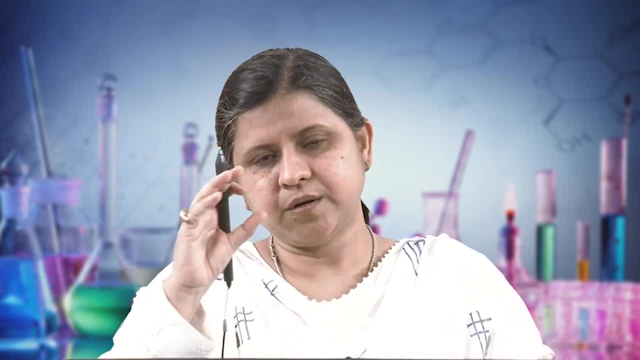 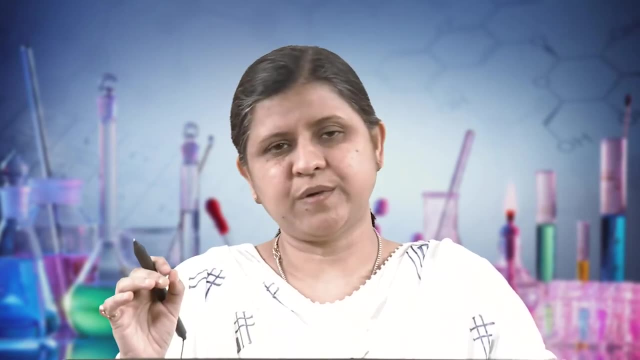 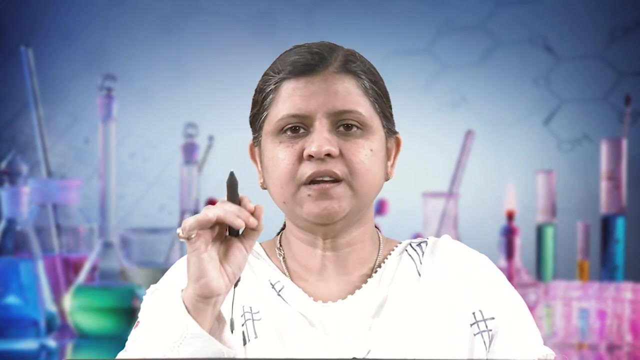 So So the diameter of two concentric pipe is not very large. okay, The diameter of two pipes are small. and if I am considering very high pressure- okay, very high pressure- then the double pipe heat exchangers becomes cheaper in comparison to. 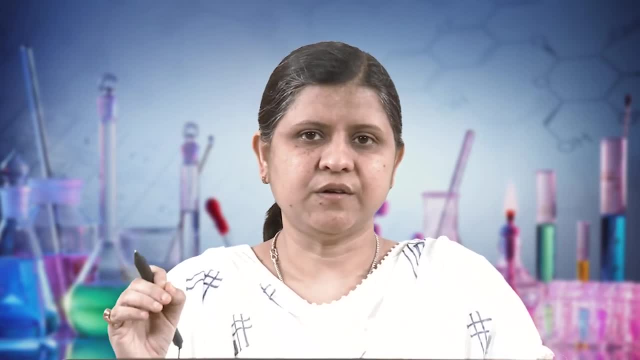 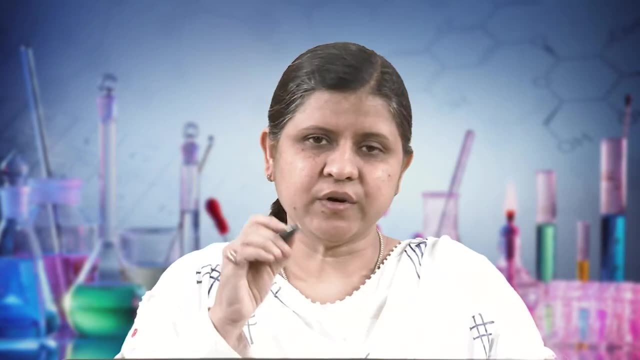 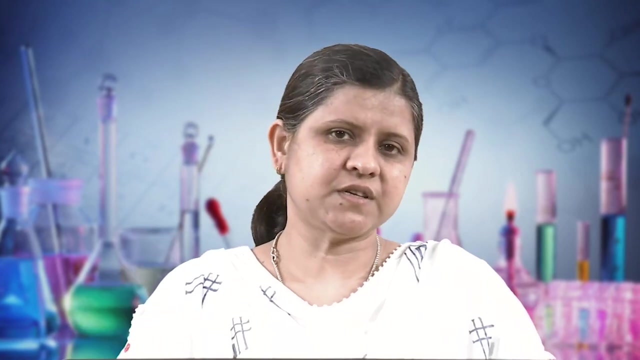 other heat exchanger, like shell and tube heat exchanger. okay, And the reason is very simple, Because what will happen when I am considering high pressure? accordingly, I have to choose the thickness of the shell or thickness of the tube. okay, Now, if I am considering thickness of the tube, how I can compute that? it can be computed. 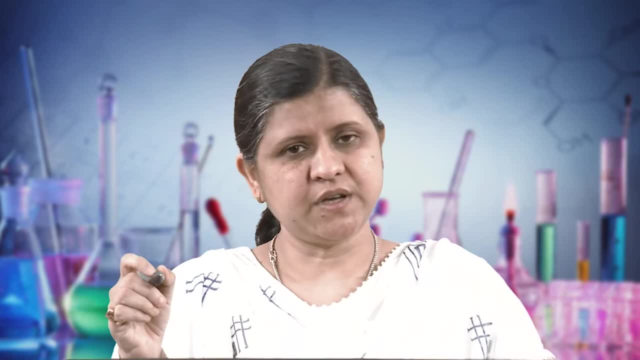 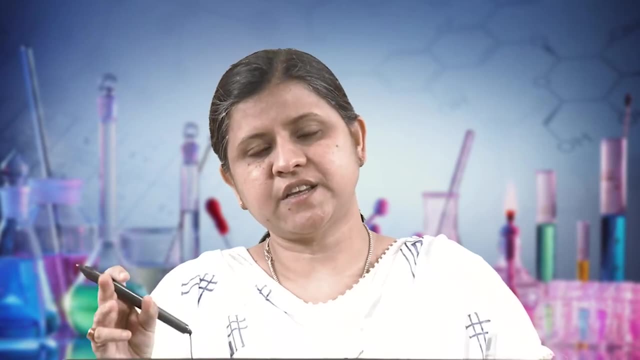 using the expression like T should be equal to P, D0 by 2 Fj plus P. okay, That is the expression. that is the expression you can consider in mechanical design. okay, So that is the expression you can consider in mechanical design. okay. 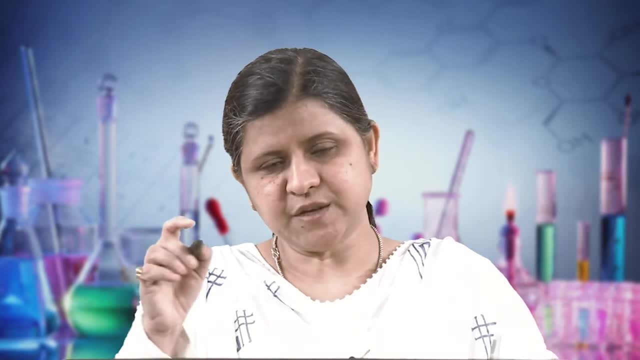 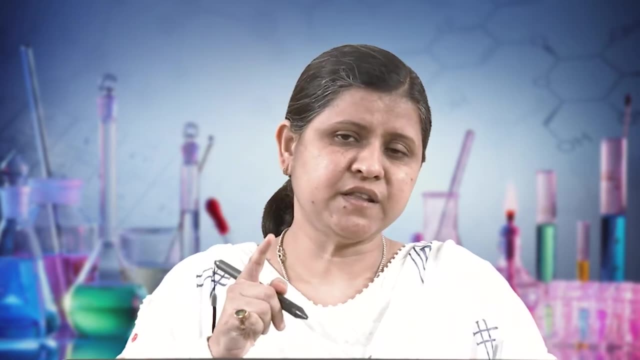 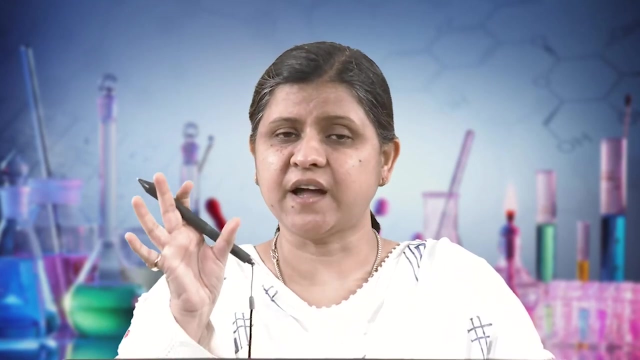 So that is the expression you can consider in mechanical design. okay, So as the pressure increases, okay, thickness will increase, fine. Along with this, there is another important parameter: is the diameter? okay, So for very high pressure, if I am considering diameter to be very large, it will consume. 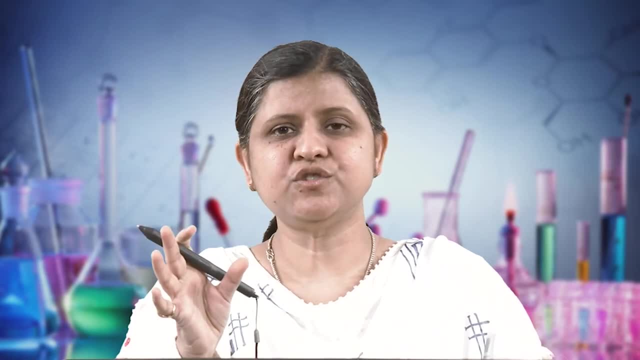 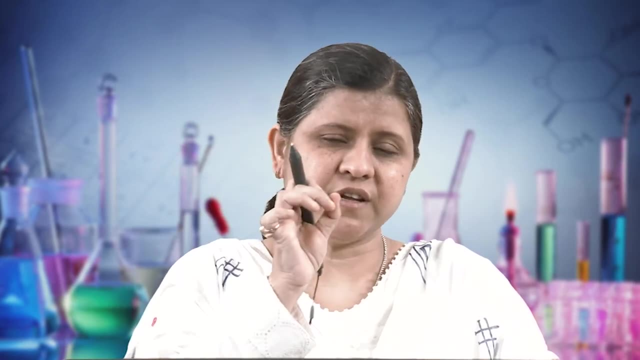 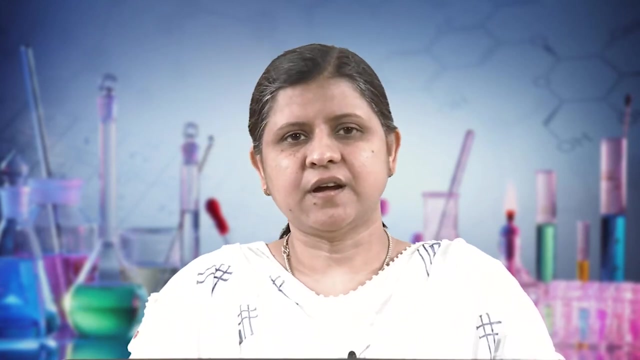 very. it will consume sufficiently large material in comparison to a small diameter, because small diameter will give less pressure. Okay, It will give lesser thickness and large diameter will give larger thickness. So obviously when I am having high pressure, so obviously when I am dealing with very high, pressure. it means we have to reduce the size of the pipe. Size of the pipe means diameter of the pipe. So instead of including high pressure in shell and tube heat exchanger, we prefer to include high pressure in double pipe heat exchanger, because diameter is small. 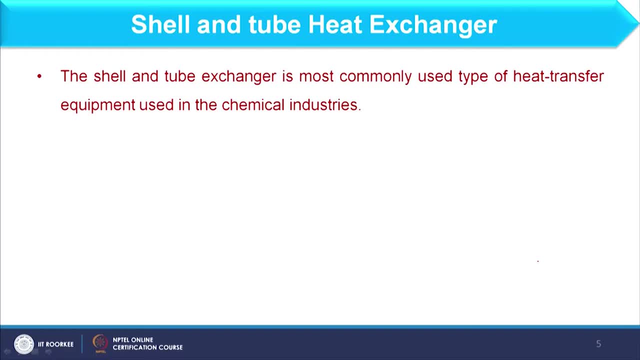 Okay, Now next unit we have is the shell and tube heat exchanger. This is the most commonly used type of heat exchanger equipment used in a chemical plant. okay, So that is most commonly used. It consists of bundle of the tube enclosed in a cylindrical shell. 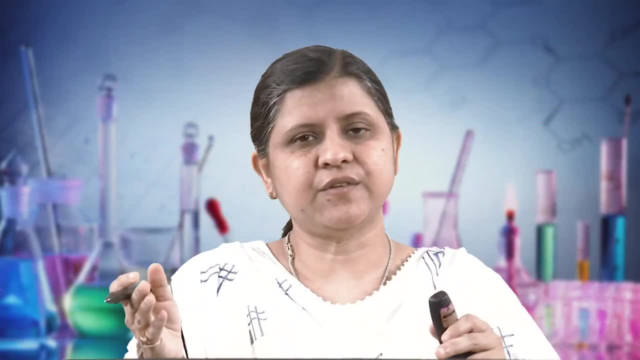 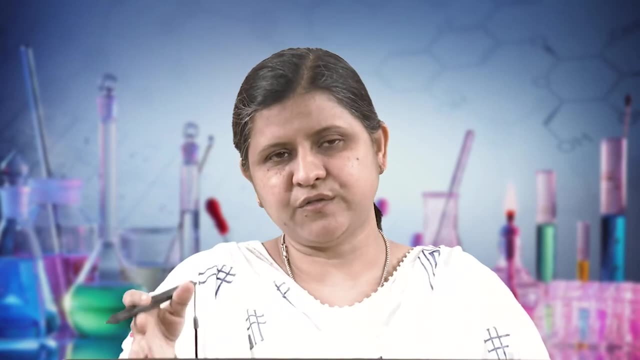 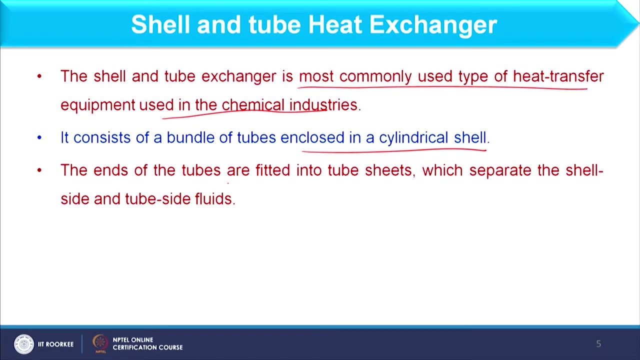 So usually in shell and tube heat exchanger, you are aware with that that it has a single shell where we have number of tubes inside this, Okay, And that number of tubes. we call that as tube bundle. So ends of the tubes are fitted into tube sheet which separate the shell side and tube. 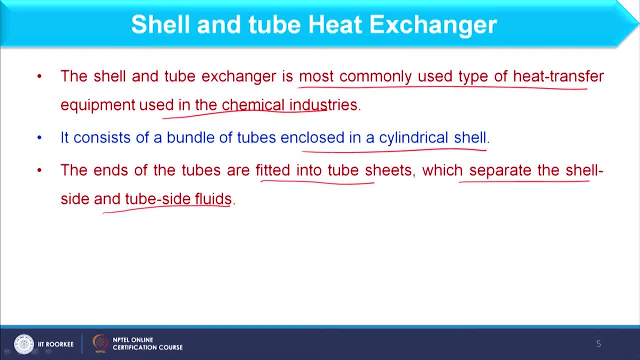 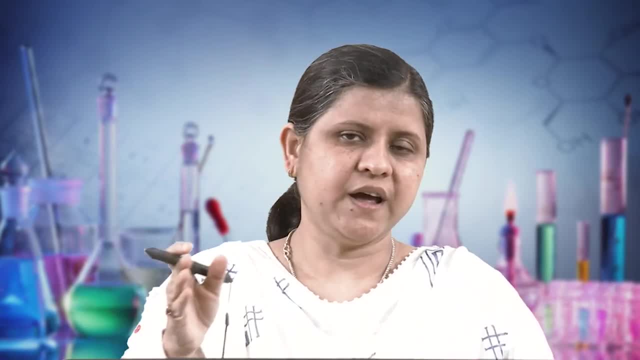 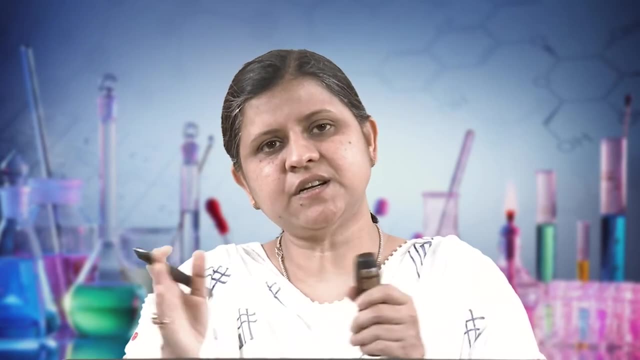 side fluids. Okay, So what will happen over here? that we have to separate the fluid which is available in shell side and which is available in tube side, and that separation is done through the tube sheet. Okay, Tube sheet has two purpose. First is it inserts the tube inside this. okay, 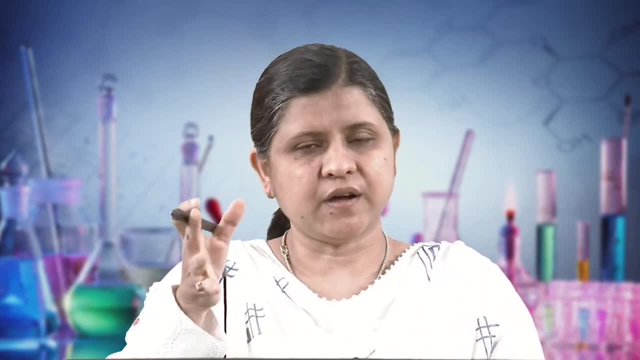 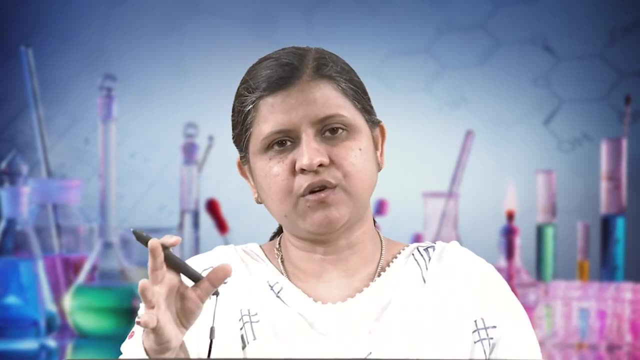 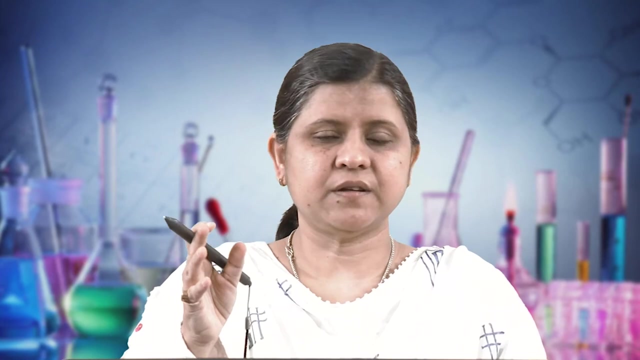 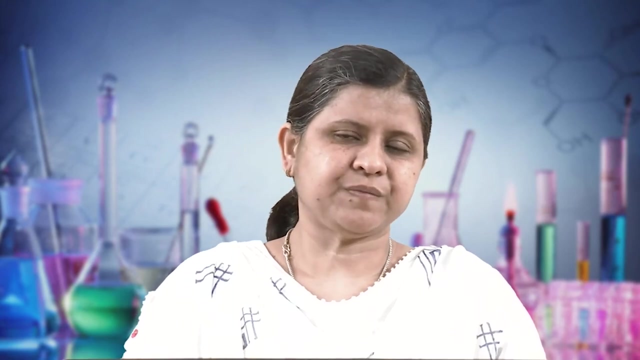 It lets the tubes inside this, okay, So it basically holds the tube from two ends. fine, And this complete assembly we call as tube bundle. okay, There are different. other assemblies are there which there are different. other accessories are there which are included in bundle that we will discuss later on. okay, 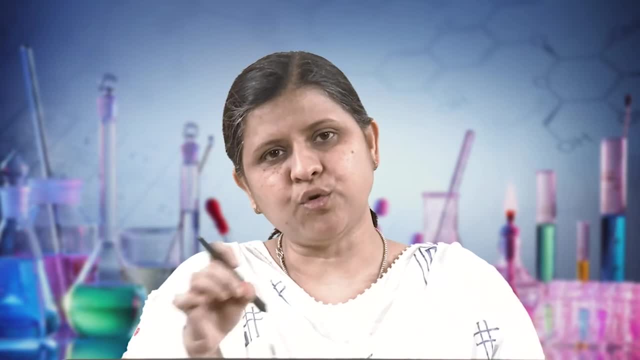 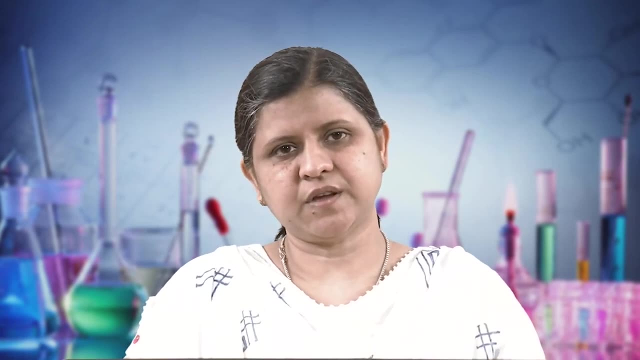 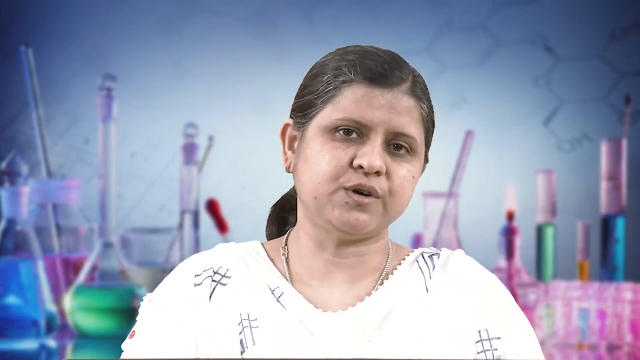 So that tube sheet, one purpose is that it basically holds the tube and second is it separates the liquid which is flowing in shell side and tube side. okay, And this point will be more clear from next slide when we will discuss the shell and tube heat exchanger through schematic. 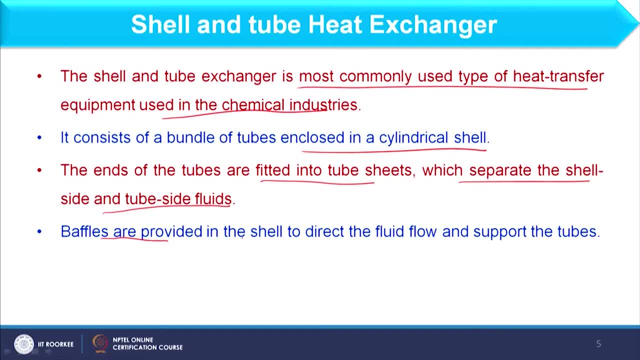 And further. we are using baffles- Okay, And these baffles are provided in shell to direct the fluid flow and support the tubes. okay. So what will happen when I am considering that tube sheet is basically holding the tubes, but it holds the tube from two ends only, okay? 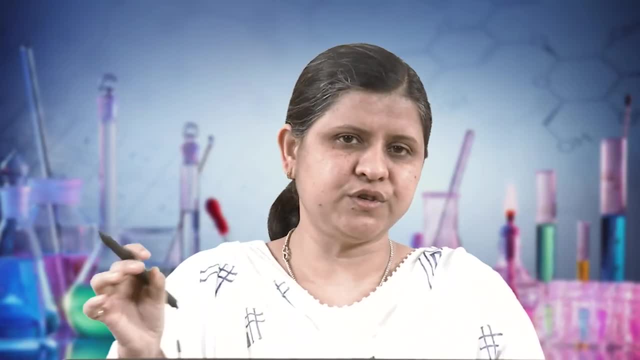 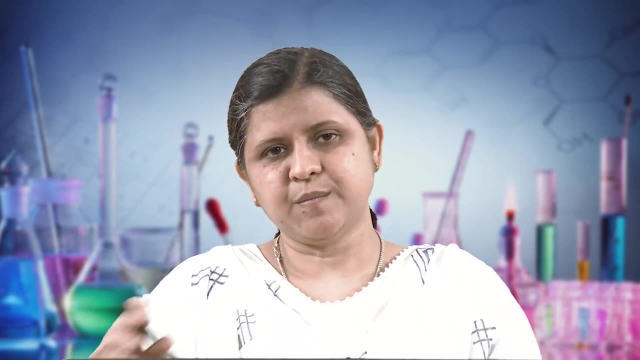 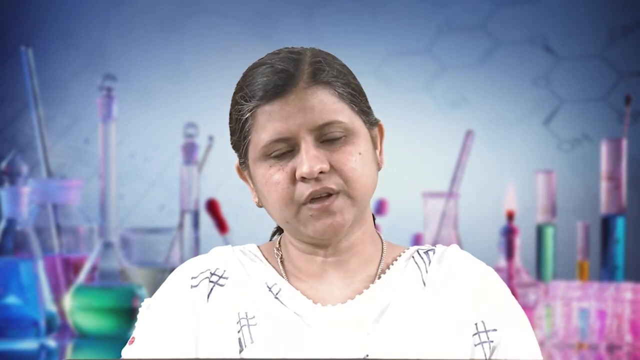 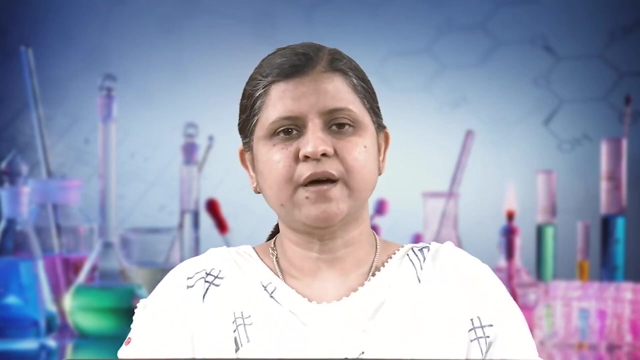 However, if we let the tube hanging between two tube sheets, what will happen? because of high velocity, vibration may occur in the tubes. okay, Because of these vibration, tubes may coincide. Okay, In the shell. okay, So to separate that tube or to hold the tube in between. to support the tube, we use baffles. 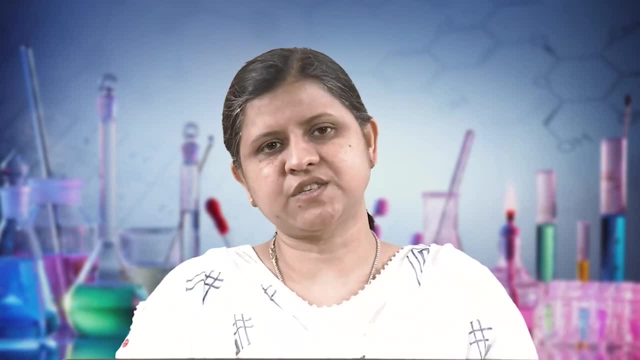 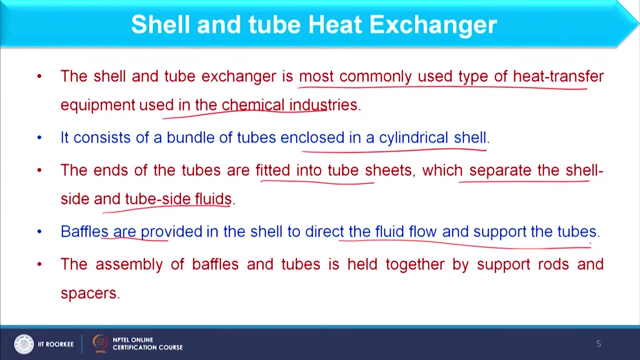 And baffles purpose is also to direct the fluid in a shell side. okay, So that I hope you understand. So the assembly of baffles and tubes is held together by support rods and spacers. So, Okay, Okay. So what is support rods? 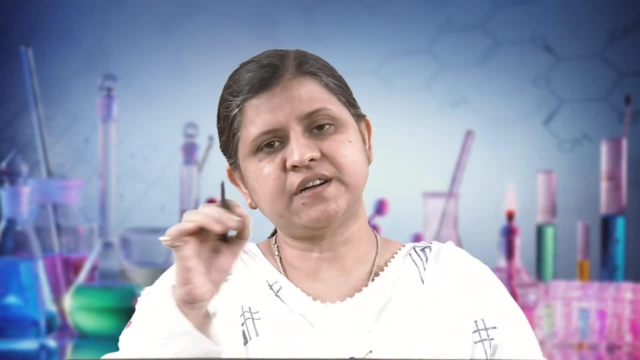 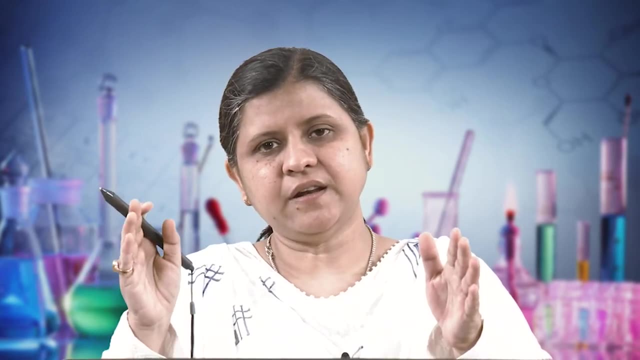 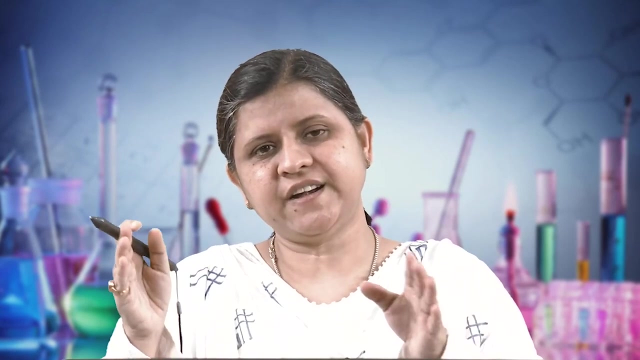 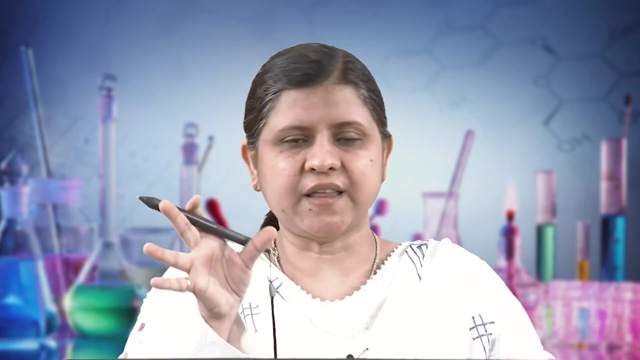 Okay, Support rod is basically the rod which is inserted in the tube sheet. okay, And that rod also contain spacers. Spacers are what Spacers are basically used to provide definite space between the baffles. okay, Because baffles are usually arranged at definite space, and that space we provide through spacers. 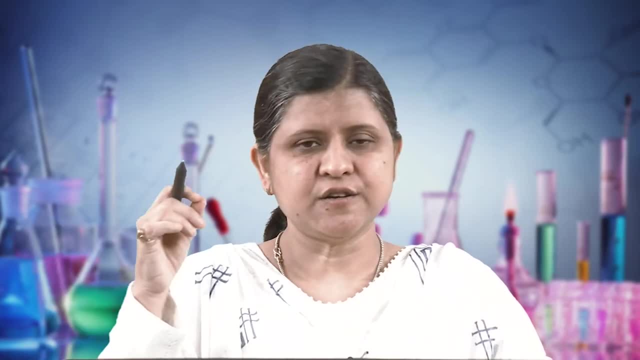 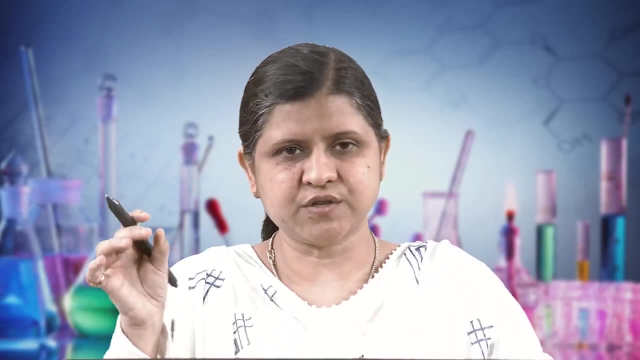 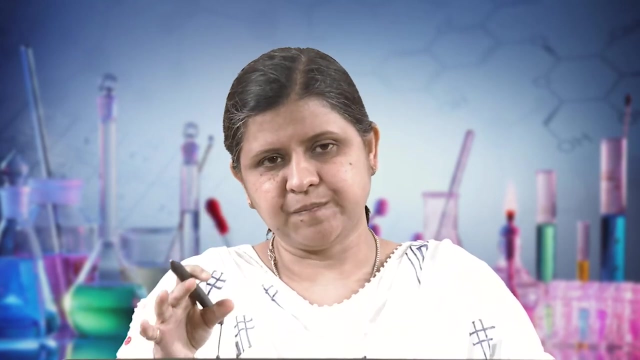 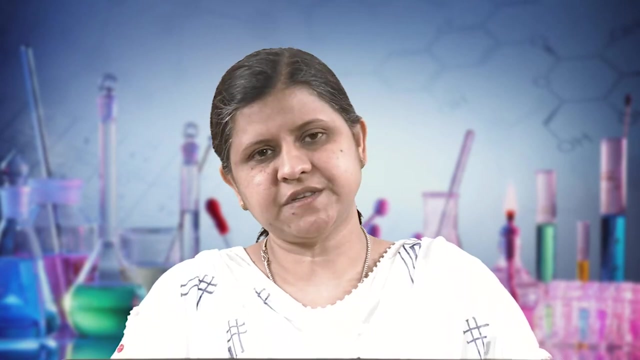 Okay, So those spacers are inserted in tube and those spacers are inserted in rods, not the tubes. okay, Because tube, if it will be inserted in the tube, so from where heat transfer will occur, So tube will remain open. and those spacers are inserted in tube and those spacers are. 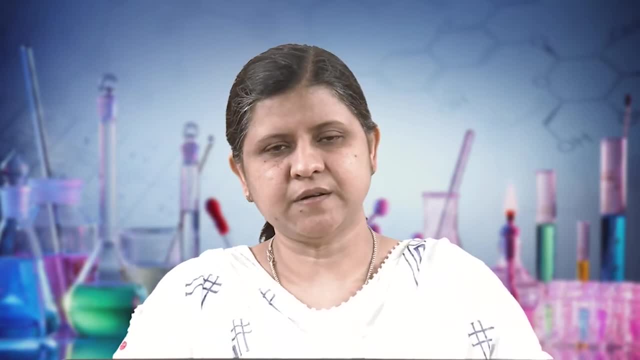 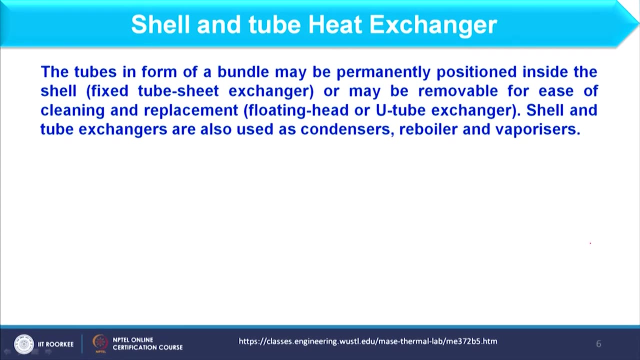 inserted in rods. okay, I hope it is clear. Okay, So, as for a shell and tube heat exchanger is concerned, the tubes is form a bundle which may be permanently positioned inside the shell. okay, So, when the tubes are permanently fixed inside the tubes, this we call as fixed tube sheet. 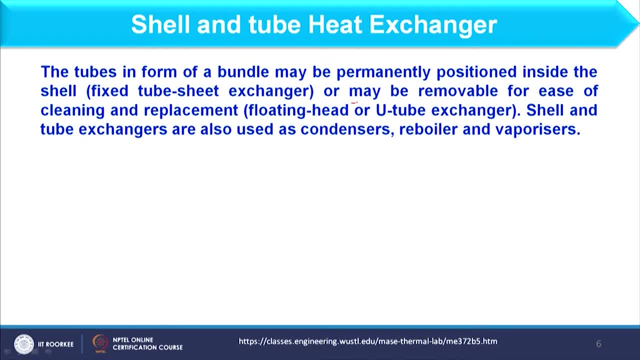 okay, And when and in some cases, tubes may be removable for ease of cleaning and replacement, and this we call as flooring, Floating head or U-tube exchangers. okay, So usually fixed tube sheet are sometimes permanently fixed with the shell and sometime 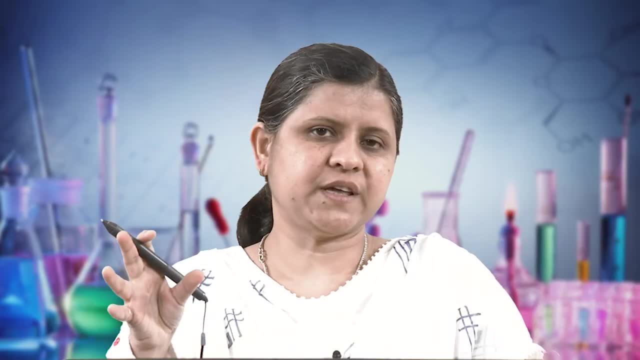 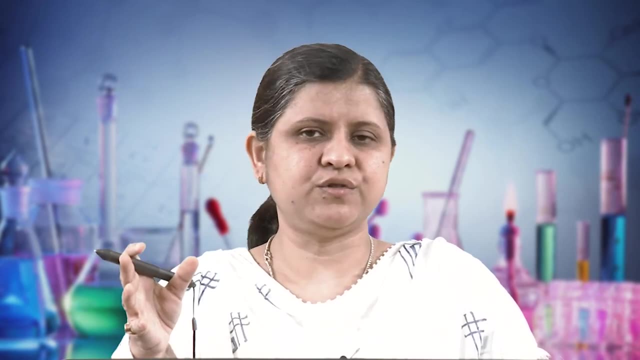 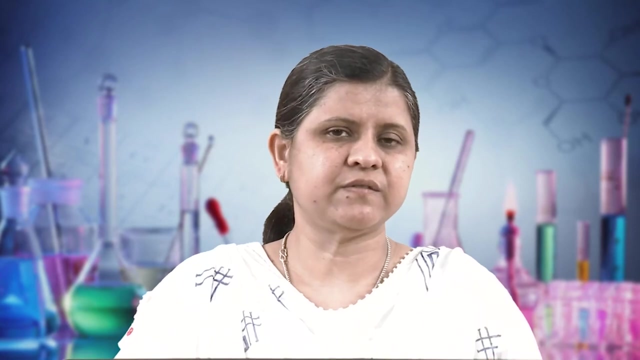 it is movable also, But in most of the cases for cleaning and maintenance purpose, it is movable So that we consider as floating head or U-tube exchangers okay. And floating head comes with a different aspect and that aspect we will discuss when we will. 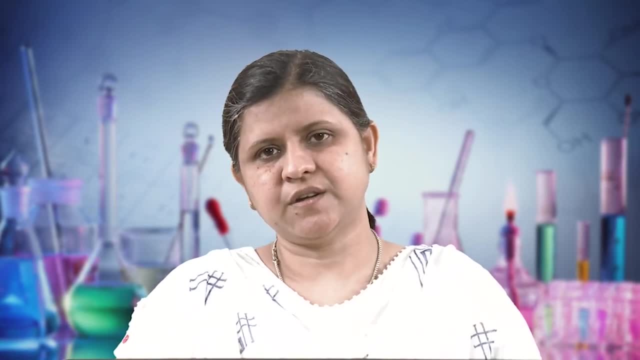 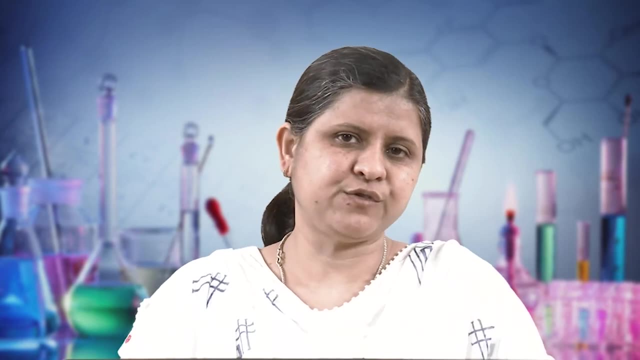 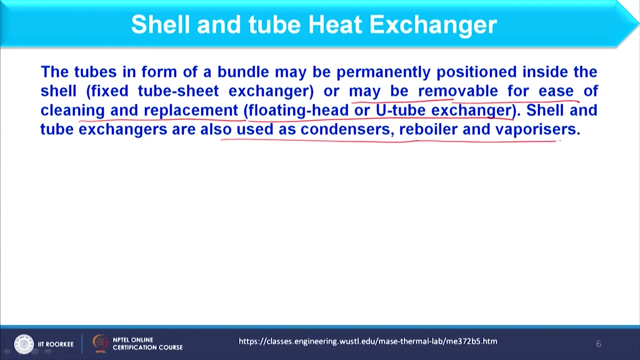 further classify shell and tube heat exchangers. okay, So it will come before design of shell and tube heat exchangers. So there you can understand the purpose of floating head or U-tube exchangers. okay, So shell and tube heat exchanger are also used as condenser, reboiler and vaporizers. 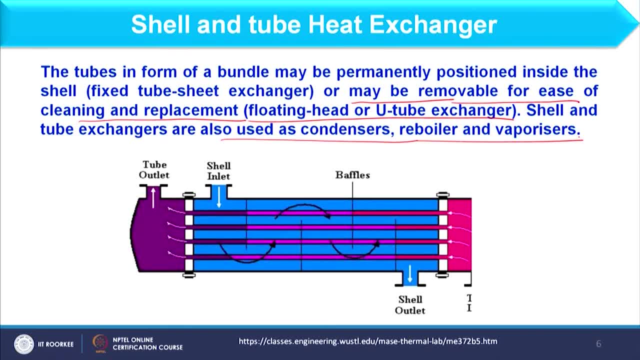 So these are some uses of shell and tube heat exchangers. Now here, if you see, we have the schematic of shell and tube heat exchangers. details you can find from this link. and here you see we have this tube sheet. okay. 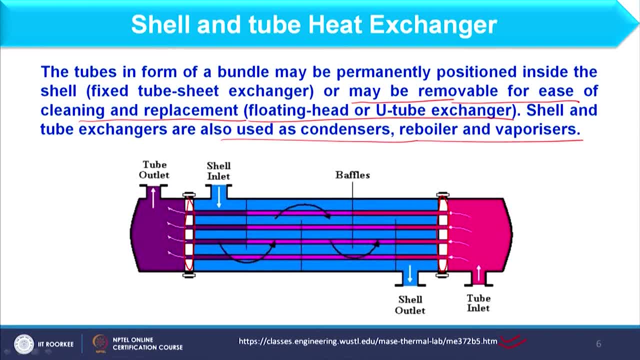 So these are basically the tube sheets at both side of the tubes where tubes are inserted. okay, where tubes are inserted as you can see here. okay, Now what will happen? this tube sheet separates the fluid which is moving in the shell. okay, 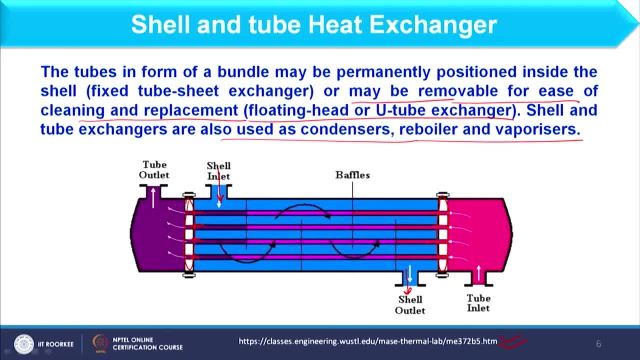 Shell inlet is here. Exit shell nozzle is here, So you can see whatever fluid is moving in this shell. it will not interact with that available in tube side, because tube side inlet pipe is there and outlet pipe or outlet nozzle is here. okay. 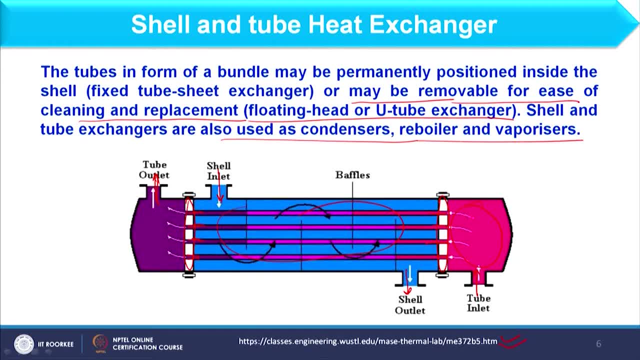 So you can see the tube sheet. purpose is to hold the tubes as well as to separate the liquid of shell and tube side. okay, Now. next is we have these buffers. Okay, Some part of the baffle is removed so that liquid can move. 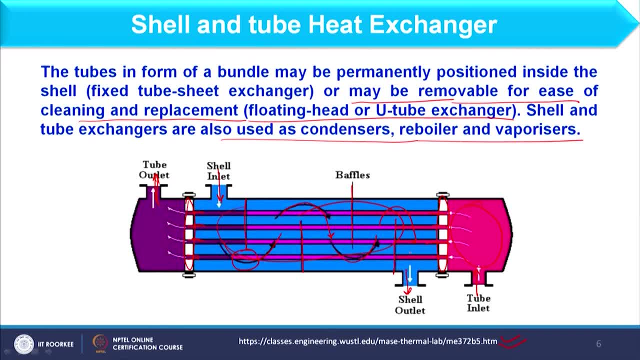 So these baffle basically provides the movement of the liquid in the shell side. along with it holds the tube. because in the pattern tube sheet has holes, in the same pattern baffle will has the holes So that tube can be inserted, Or Okay. 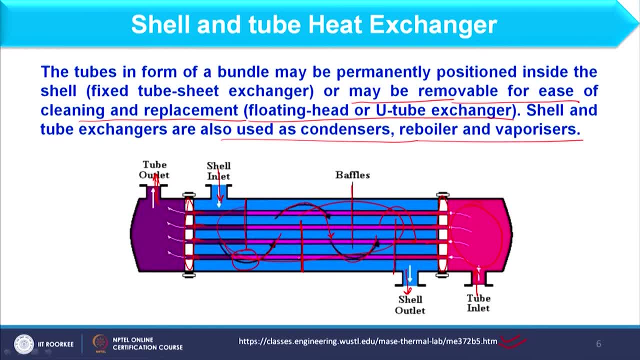 tube can be inserted in the baffle. okay, So when I am considering tube bundle, tube bundle basically includes this tube sheet, these tubes, baffles and rods. So where rod is attached, Rod is attached like this here. okay, This rod is not the part of the tube. okay, and how? 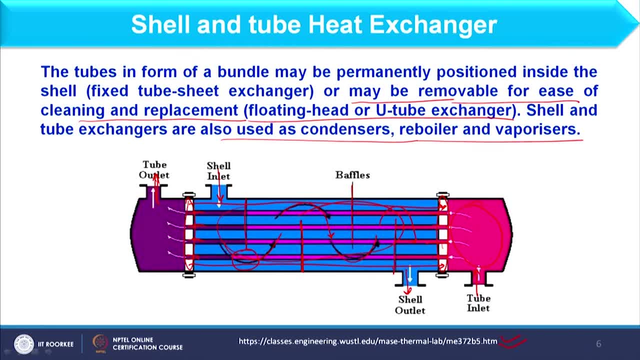 this rod looks like. it is like you must have seen, like TMT bars. okay, So this tube is like. so this rod is like TMT bar where spacers are provided, like if I am considering this space between baffle and tube sheet. so first spacer will insert and then baffle will insert. 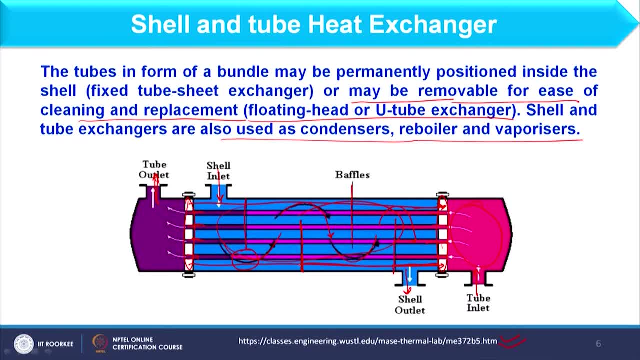 Then again we provide the spacer and then the baffle. okay. Similarly, tube bundle In this side- okay. So in this way we put the spacer in rod and then we insert the baffle. So this is assembly for shell and tube heat exchangers. We will further discuss these. 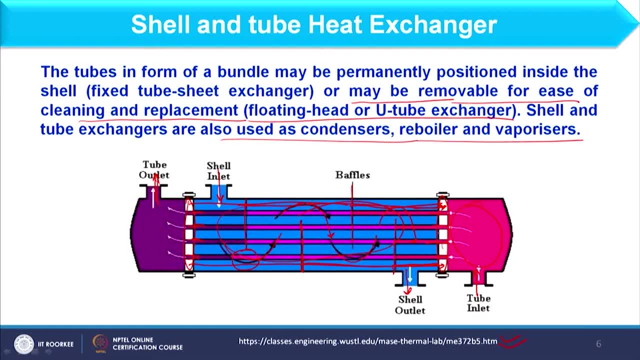 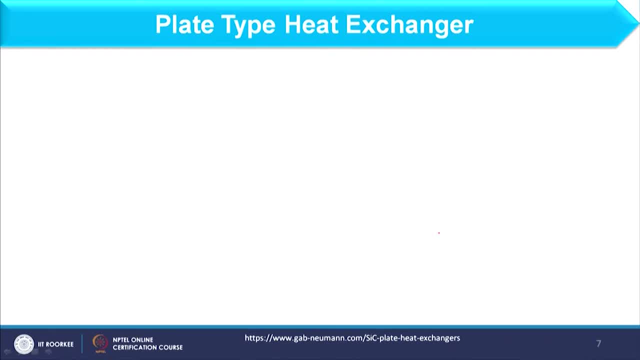 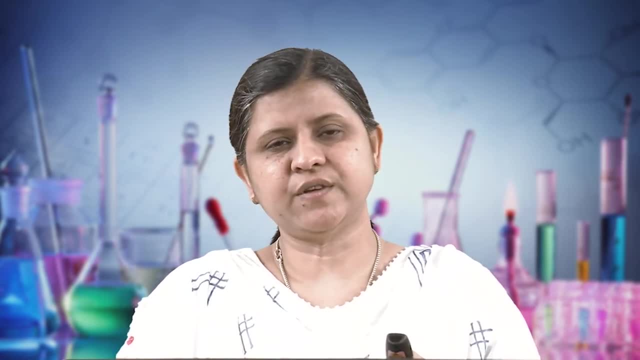 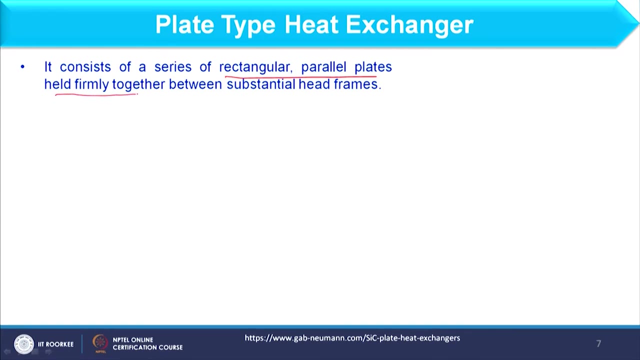 each accessory when we will cover the shell and tube heat exchanger design. Now let me focus on plate type heat exchangers. okay, As we have tube and shell in shell and tube heat exchangers, here we are dealing with the plates. okay, So it consists of series of rectangular parallel plates held firmly. 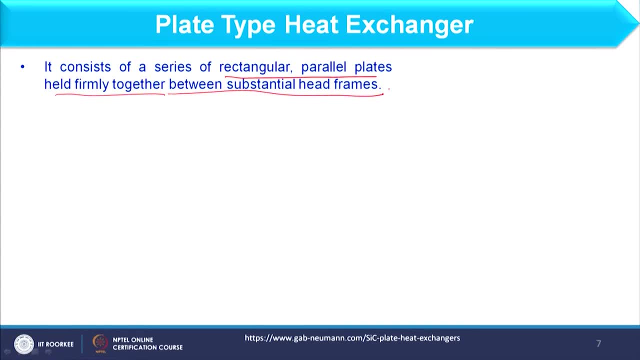 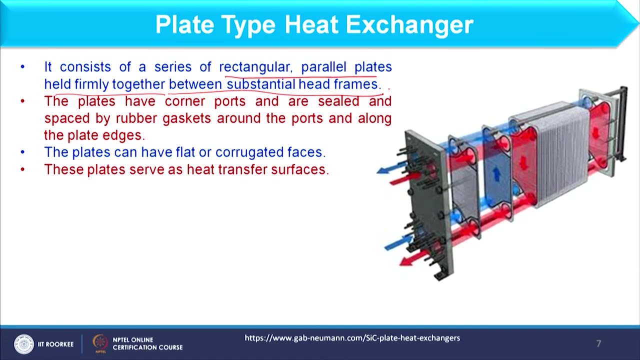 together between substantially head frame. So here you see, in plate type heat exchanger we have the head frame that I will show. okay, Slide time, Spacer height. Summary of plate type heat exchanger. Let me show that first. fine, Now, if you see this schematic, this structure, this rectangular plate and this bar and over, 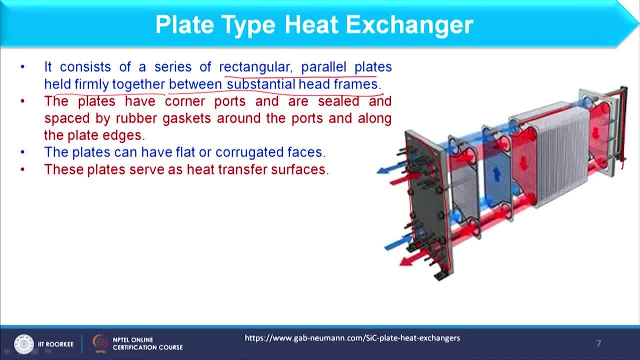 if you see, at the top we have this bar also where these plates are hanging. So this bar is available at top as well as bottom, both side, okay. So each plate type heat exchanger has plates which are arranged parallel to each other like this and this, and it is firmly together with a substantial head frame. okay, 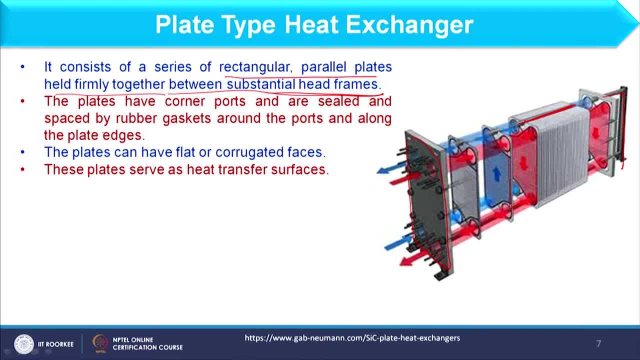 And plates have corner ports and are sealed and spaced by rubber gaskets around the ports and along the plate And along the plate edges. okay, Now, what is this? If you consider each plate, either you consider this plate, this plate, or this plate each. 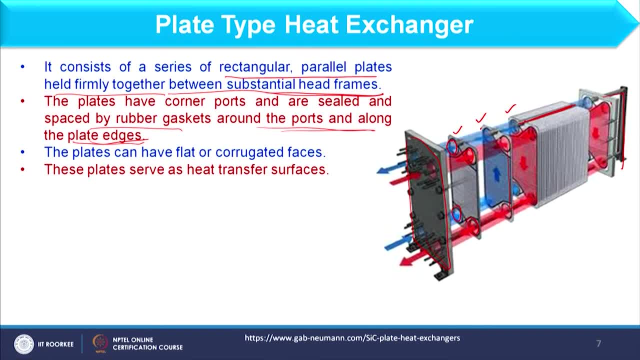 plate will have 4 corners. fine, Now what is the purpose of these corners? The purpose of these corners are it basically let the fluid enter or let the fluid pass through it? okay, So each plate will have 4 corners. And if you consider this particular plate, the second plate, here we have this black. 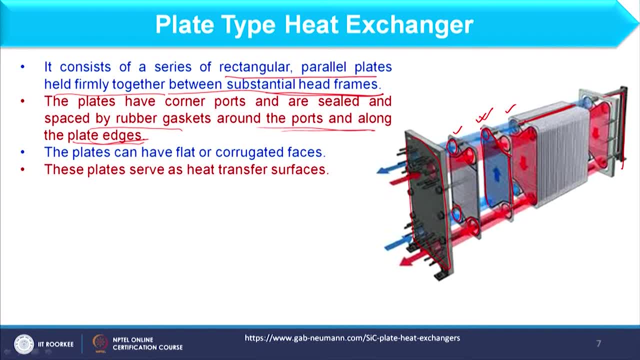 assembly. okay, Here we have this black assembly, and this black assembly is nothing but the gasket. okay, Now, if you focus on this plate, what will happen when fluid is coming? okay, And how the movement of fluid occurs over here? 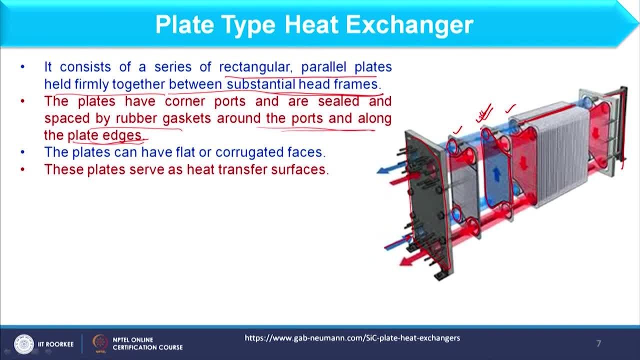 Okay. So here we have the cold fluid, fine, which enters from here and exits from here. Similarly, hot fluid enters from here and exits from here. okay, So when it is entering into the system or entering into the heat exchanger between two. 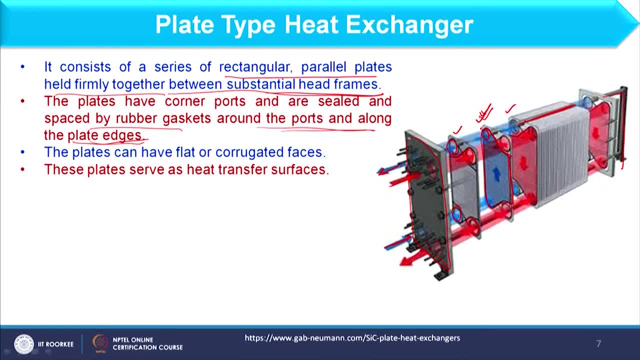 fluids. there is no fluid which can be entered in this region, because here we have the frame only. Okay. Okay, Here you can see that the film moves like a plate. This is the cold fluid which goes through as a heat exchanger plate. okay, 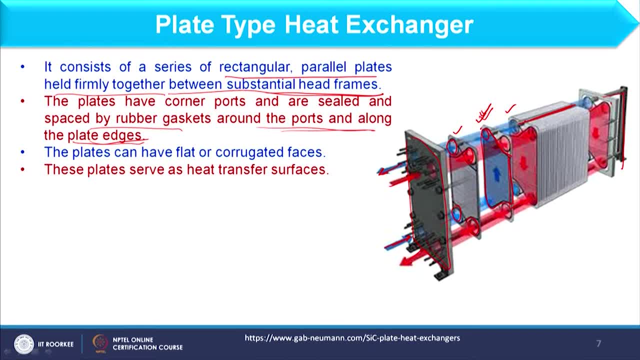 Okay. so what will happen? whatever cold fluid is coming, if you see this particular plate, here we have the gasket And gasket closes this corner and closes this corner. okay, So, whatever cold fluid is coming, it will pass over this or it will spread over this. 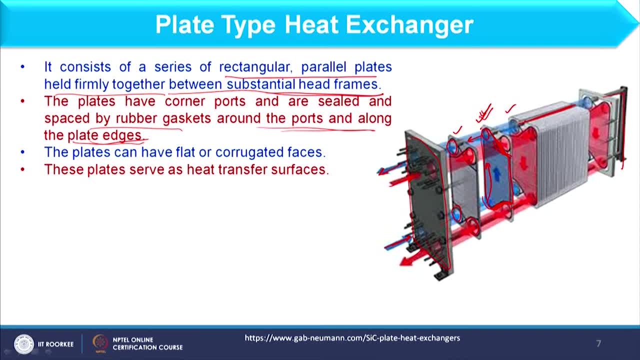 plate and exits from here because it cannot enter to this corner or to this corner. fine, It will go from here to this, So cold fluid will pass through this plate. In this case, there will not be anyWAY ACACU, okay. 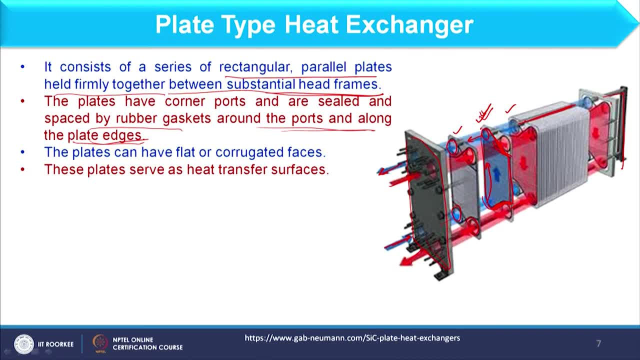 It will not go through this plate. okay, install temp drink. Okay, Okay, 1 min. Next audience In the similar line. if I consider this third plate, then what will happen? gasket is attached like this: okay, because it is putting a bar over here or hurdle over here. it will not. 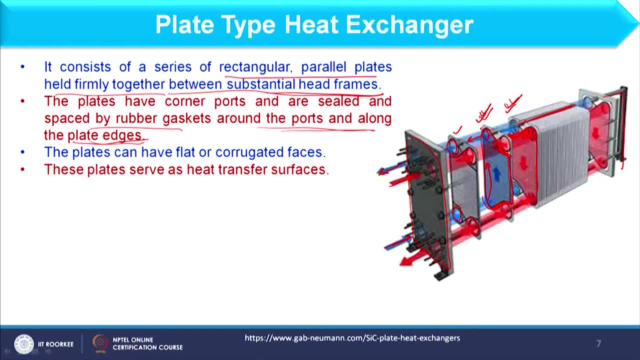 allow cold fluid to enter into this. okay, Open space is available only for the hot side. okay, So these two nozzles you can consider for hot fluid, these two nozzles you can consider for cold fluid. okay, So, because it is open for hot fluid, the fluid will come over here, spread over the plate. 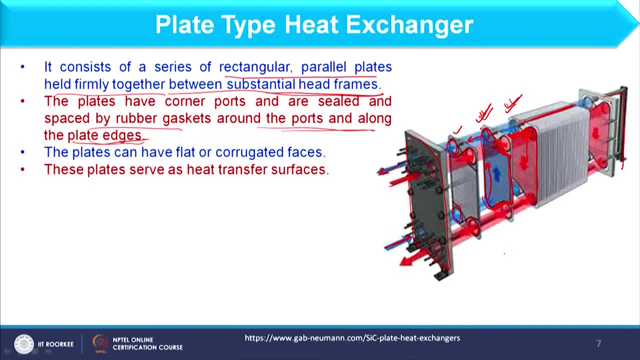 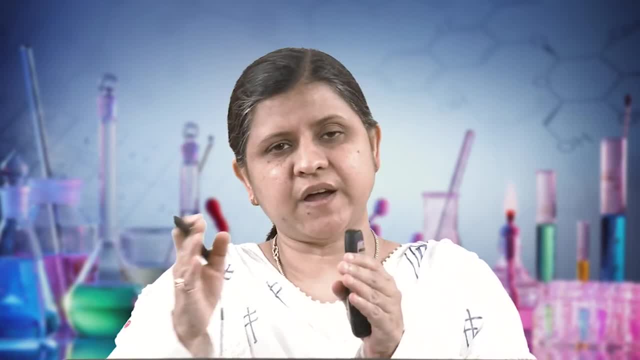 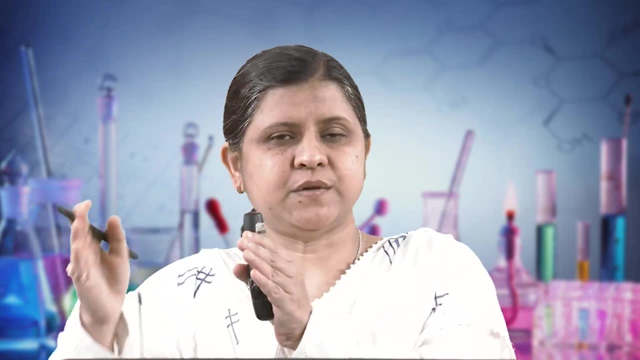 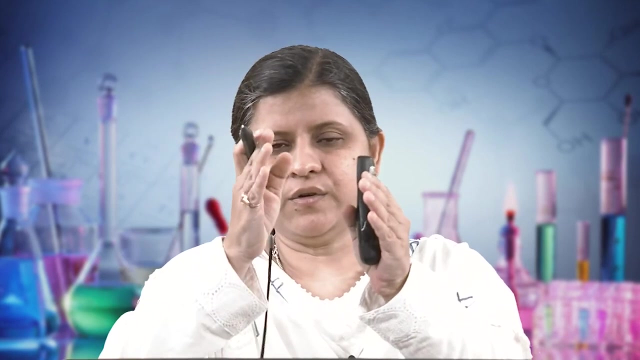 and then exits from here. okay, So all these plates are attached one by one, okay, and between two plates one fluid will move and in the subsequent side or in the consecutive side, another fluid will move, okay, So if I am having this type of these two plates here, I am having cold fluid then. 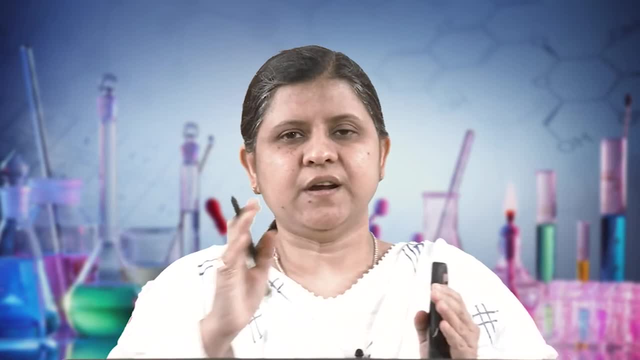 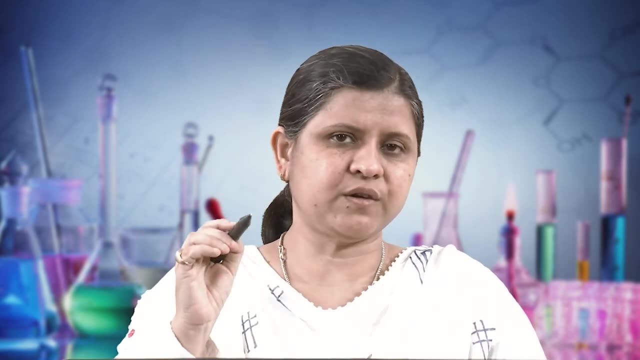 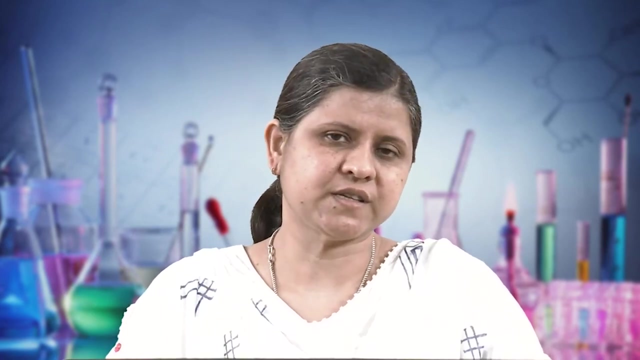 here I am having hot fluid, then cold fluid and then hot fluid, like this: it will keep on moving. okay, And how we will ensure that only cold fluid will enter and only hot fluid will enter? that is because of gasket. okay, I have already explained that how gasket is placed, so it will not allow another fluid. 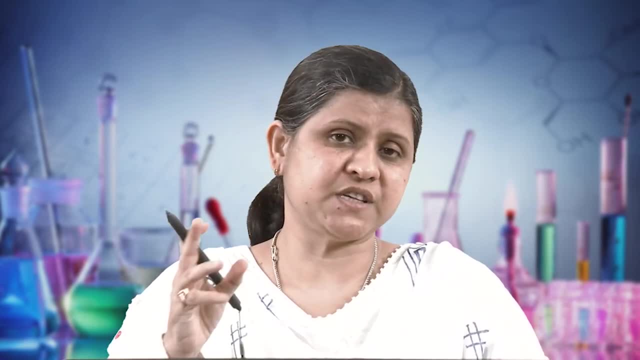 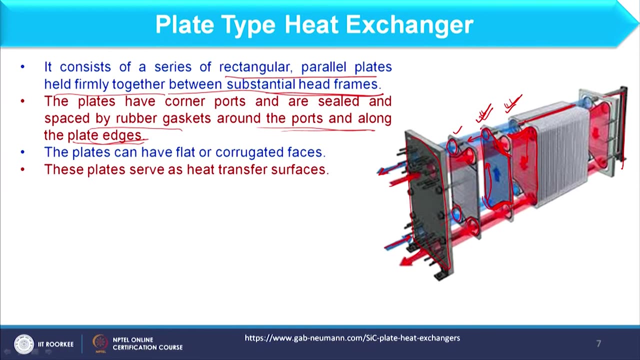 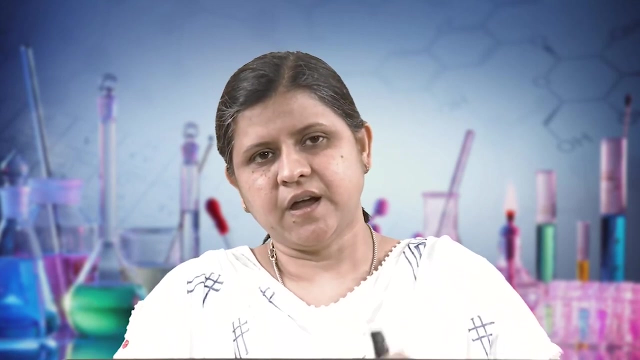 to enter into one plate. or we can say the mixing plate, Okay, The mixing of plate. or we can say the mixing of fluids on a plate, which is not possible over here, okay, So separation of fluid will occur through this gasket, okay. 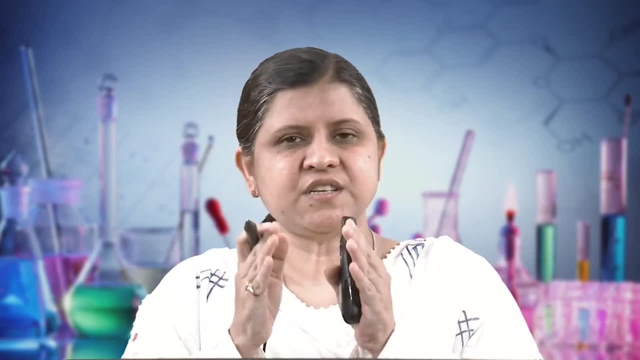 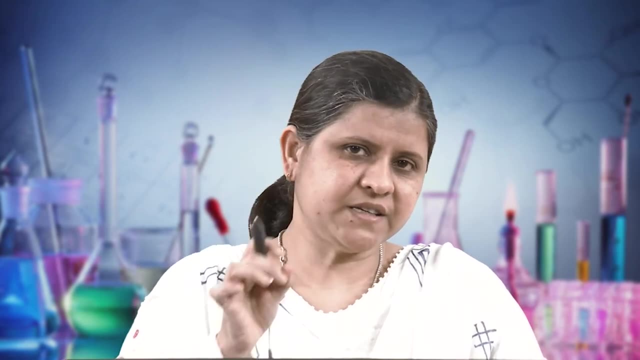 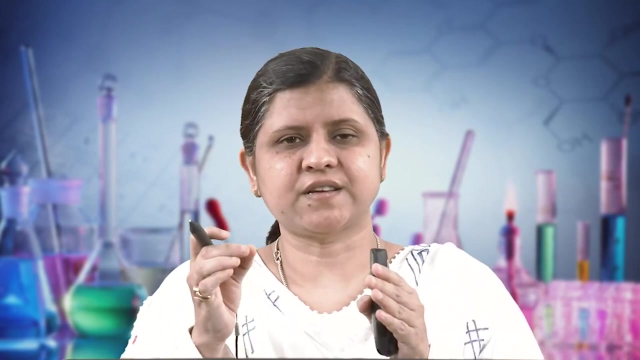 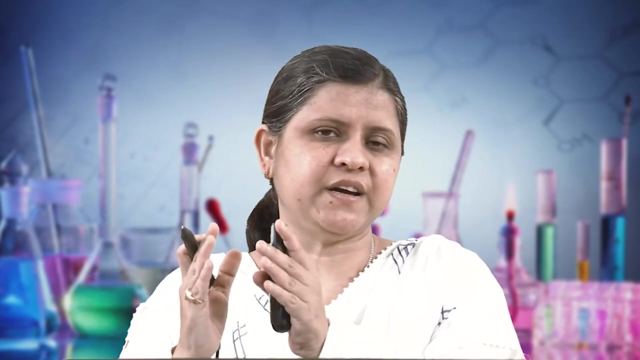 Now, what will be the distance between two plates? okay, How we will ensure the proper distance between the two plates. that distance can be according. that distance, Okay, Is according to the thickness of gasket. okay, because each plate will be placed so tightly. 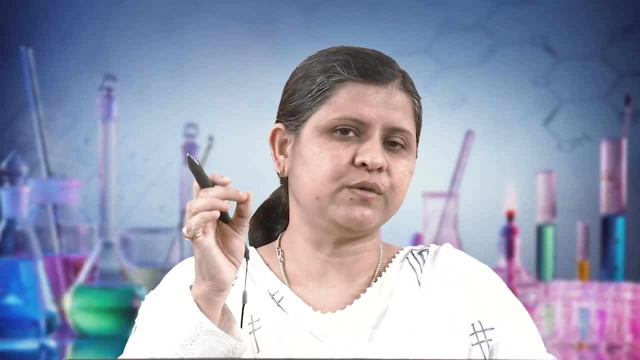 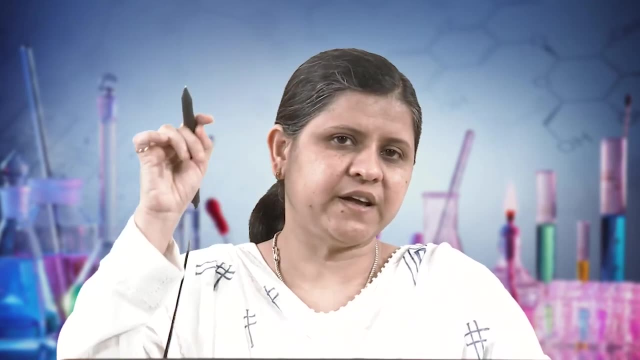 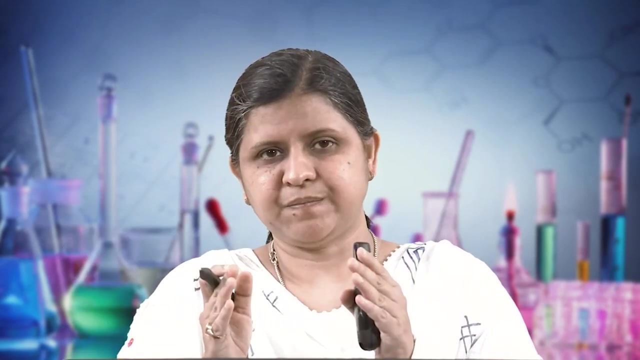 that the space between two plates will be only equal to the thickness of gasket. okay, And if I am not using that gasket, we sometime weld that particular section. So welding means what two plates will be joined permanently. welding or brazing means 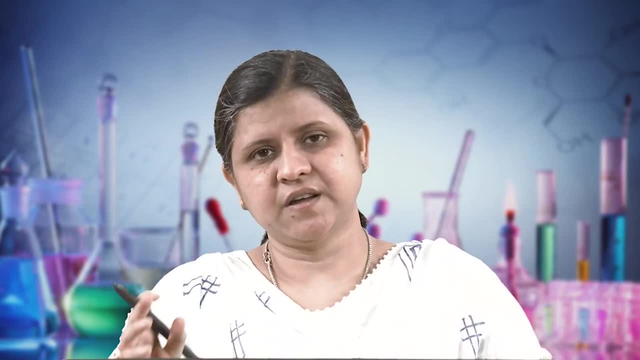 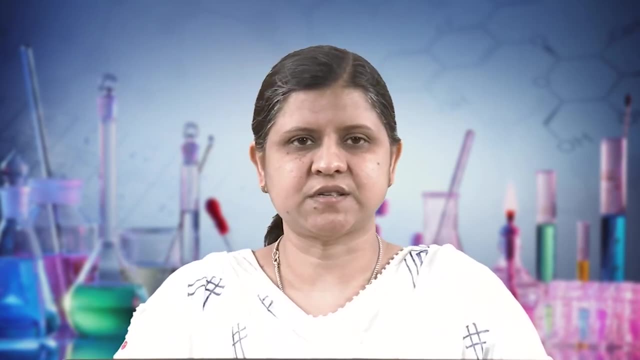 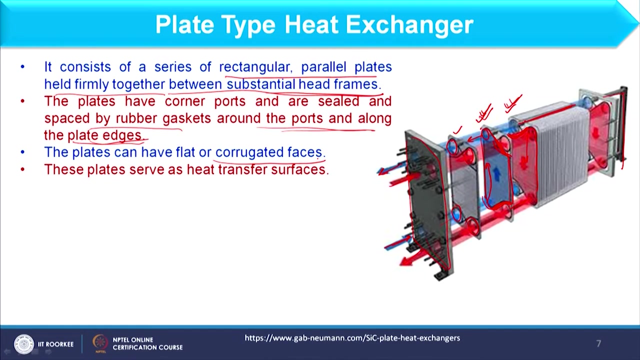 what two plates will be joined permanently. So that is, it has an advantage and disadvantage also, and some disadvantages are there with gasket also that we will discuss later on. So plates can have flat and corrugated faces because each plate will have some structure. 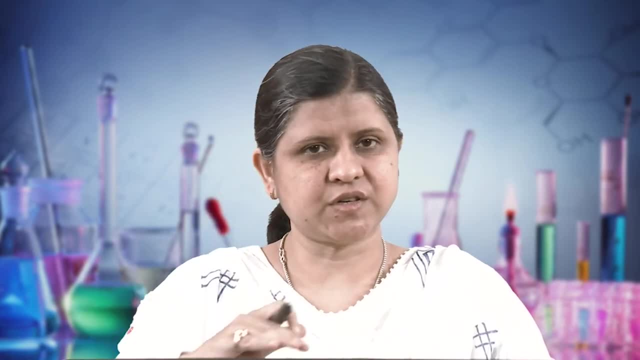 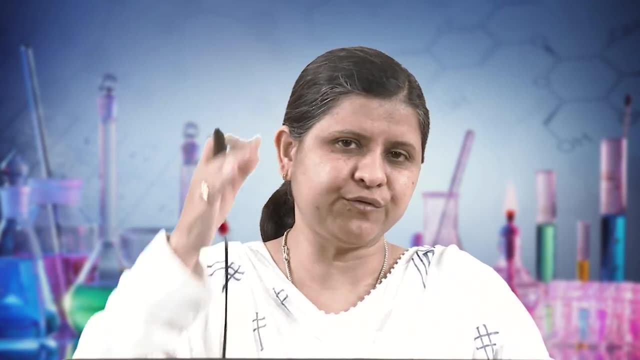 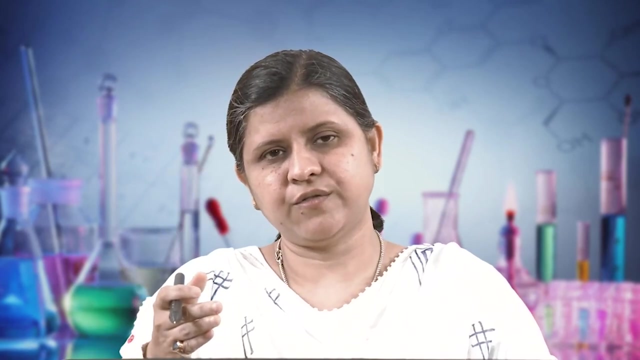 we have some depression in this. we have wavy structure also and because of this we can find more turbulence over the plates. okay, When the fluid will move because of this hazy structure, more turbulence will be found. more turbulence will be there over the plate, which increase heat transfer coefficient. 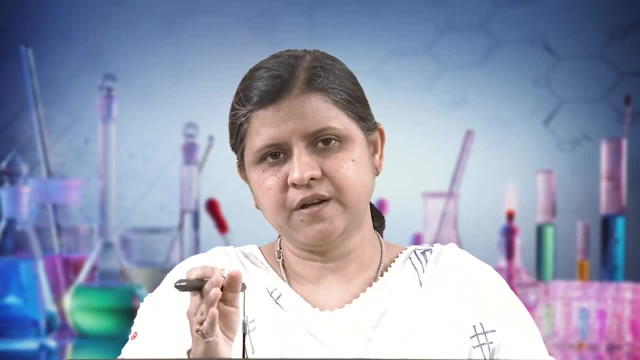 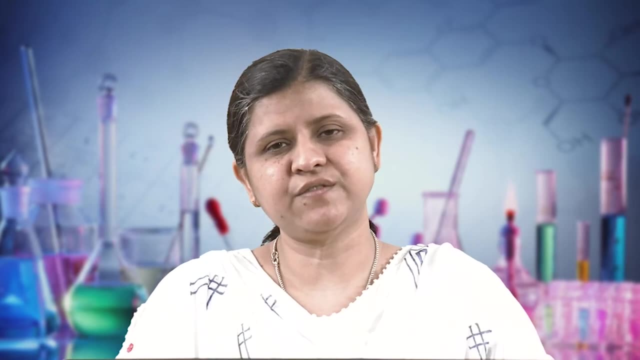 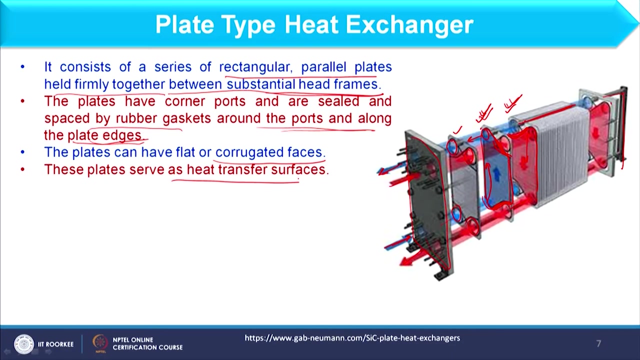 So when you compare the heat transfer coefficient of plate heat exchanger and shell and tube heat exchanger for the same heat transfer area, heat transfer coefficient will be significantly high in plate heat exchanger because of this structure only, Okay, And these plates serve as a heat transfer surface, okay. 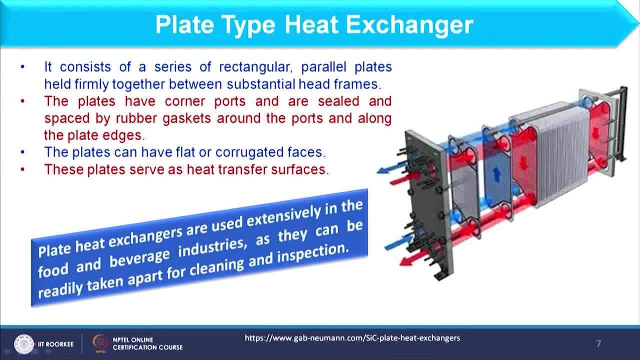 So this point we have already discussed. So, as far as utility of plate heat exchanger are concerned, these are used in food and beverage industry, as they can readily taken apart for cleaning and inspection. okay Now, as I have told you that two plates are very compact or very close to each other, okay, 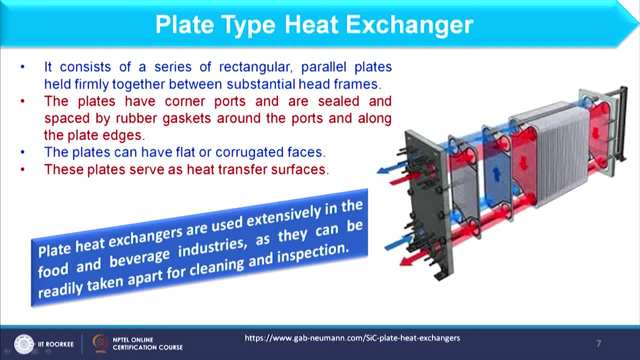 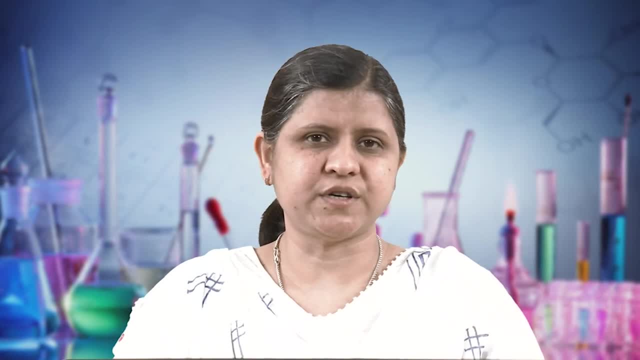 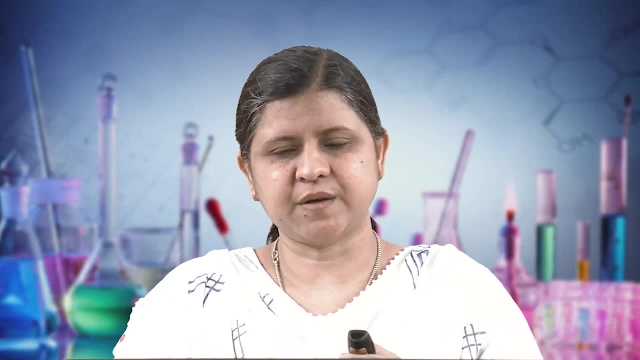 it means it has very high tendency of scaling. Okay, And to avoid that, usually plate type heat exchangers are used for clean fluids, not the fouling fluids. okay, So that is the main point about plate type heat exchanger and if you see, here we have 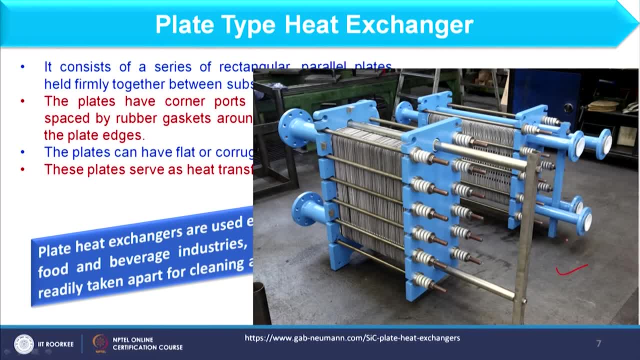 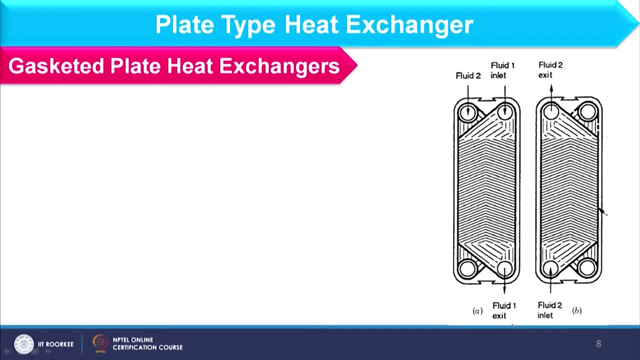 this photographic view for actual heat exchangers, and you can find details about this on this website. Okay, So that is about the plate heat exchangers. Now, here we have gasketed plate heat exchanger where we put the gasket. 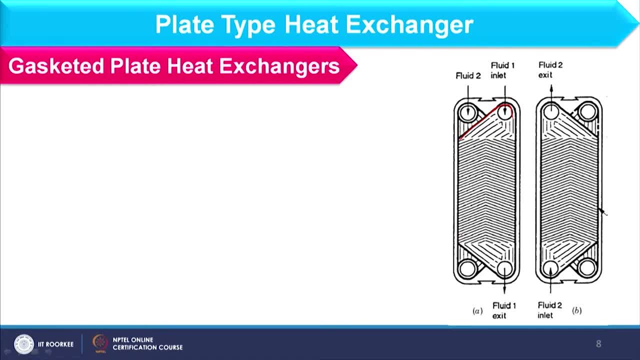 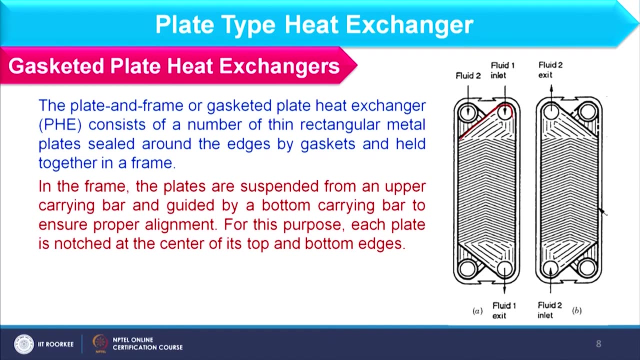 This is basically the gasket from last figure. it is more clear in this figure, So you can imagine this. you can see the gasket over here, okay, So, and if you consider this notches, okay, Here we have the notch. so these notches are basically used to hold this plates. 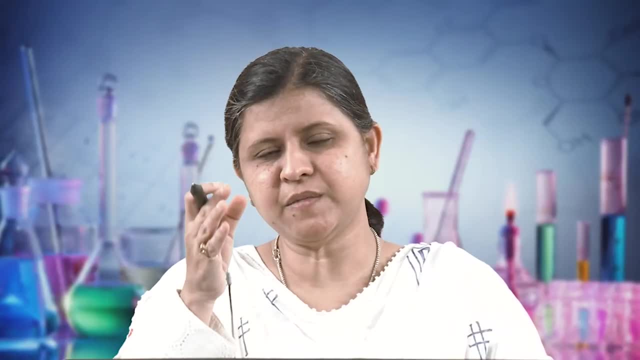 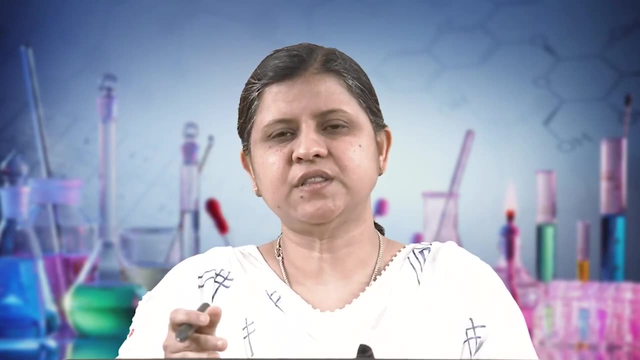 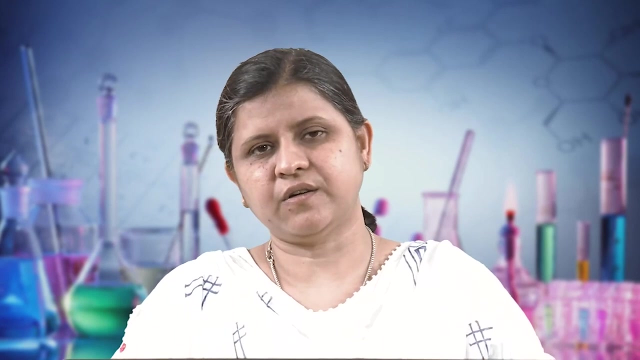 So, as I have already discussed, that frame is used where these plates are hanging. okay, So hanging means what it is basically fixed with this notches. So, wherever required, the plates can be removed, clean and further placed on it and further placed at the right. 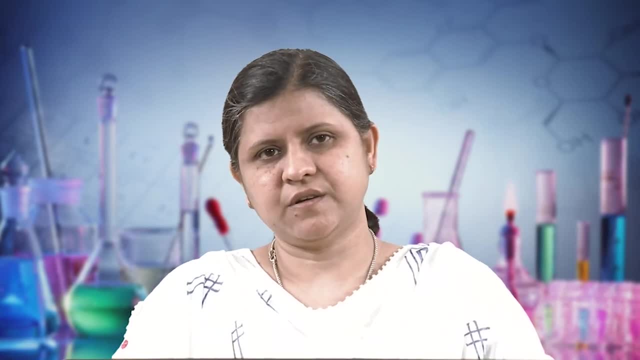 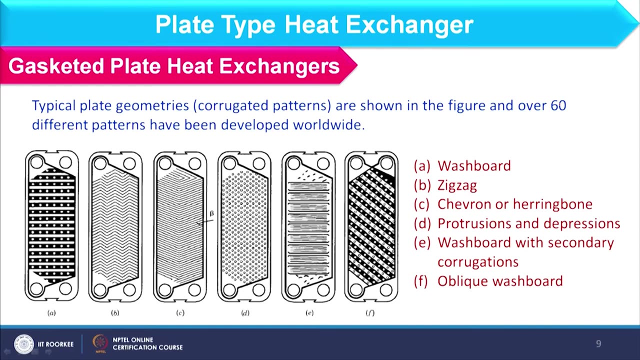 Okay. Okay, So that is with the gasket plate, heat exchangers, and here we have different types of plates. In some plates you can have this zigzag structure and in some cases this we call as Herrick bone type of structure, and washboard are also there. 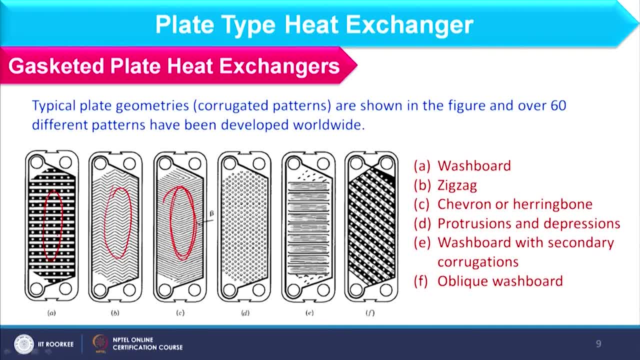 So you can see we have different types of plate and when we cover the whole total design over the plate it is more than 60 different patterns over the plate. So you can understand the structure over these plates or the pattern over these plates. 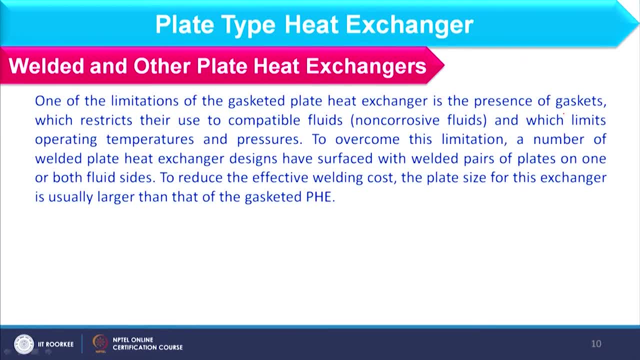 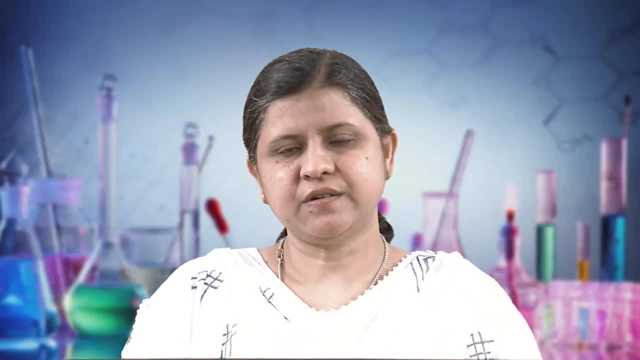 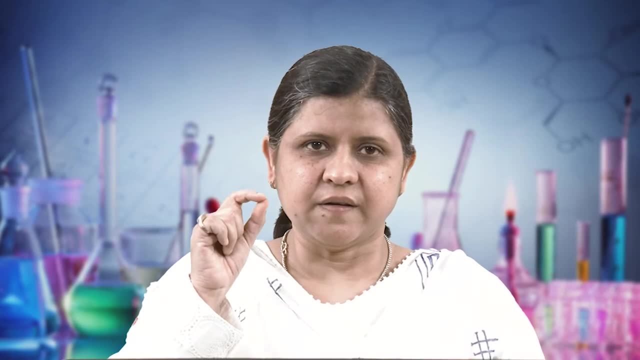 Now we will discuss welded and other plate heat exchangers. So first of all, now tell me what is the limitation of gasket plate heat exchanger? Okay, The material of gasket is usually rubber type, fine. So we cannot handle very high temperature or very high pressure fluid in such type of. 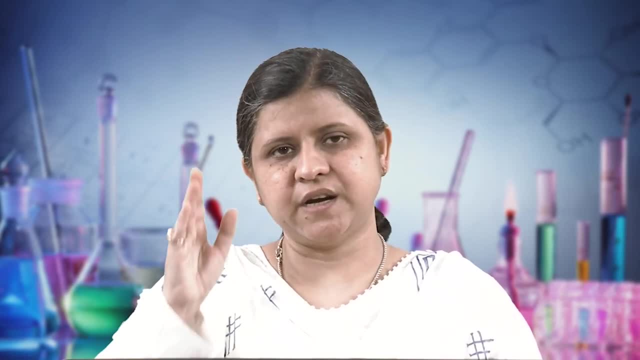 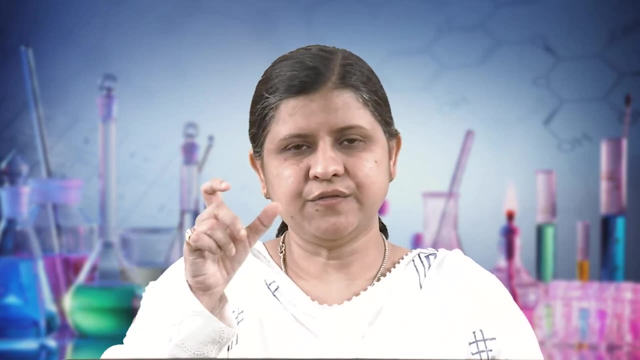 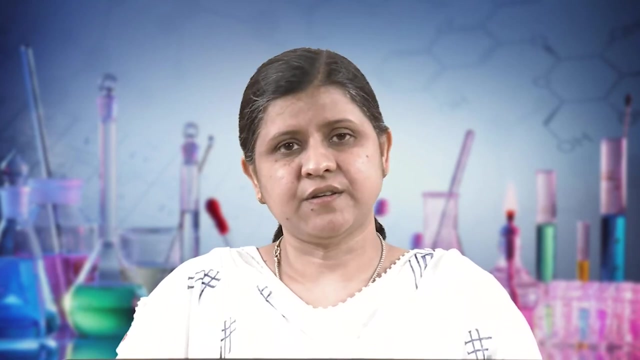 heat exchangers when I am using the gasket, because gasket will tear and fluid may come out. okay. and if I consider further, because reaction of fluid with the gasket material is significantly high in comparison to welding or other type of structure, okay. 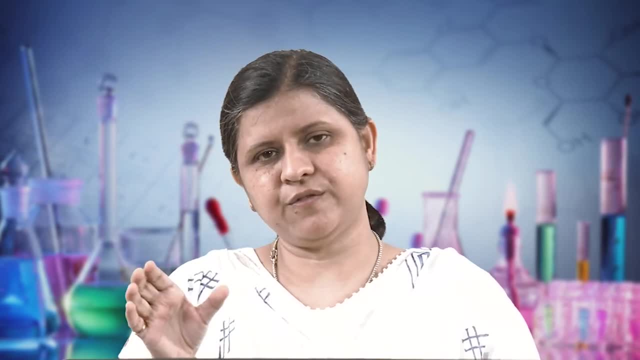 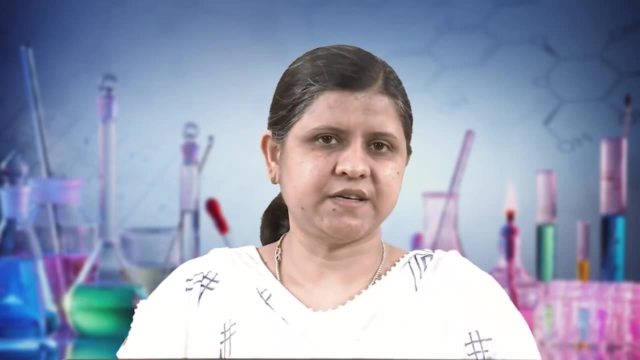 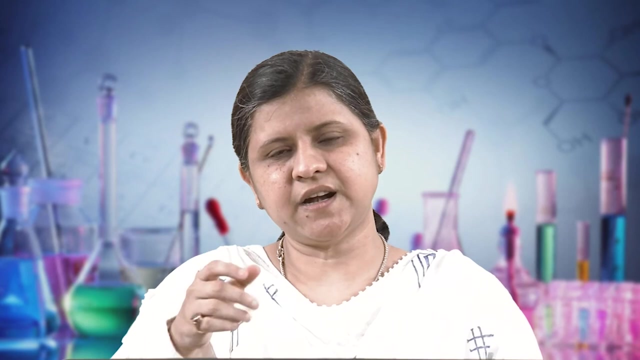 So that is basically the limitation. So where I am having this type of condition, I basically weld the two plates together instead of gasketing it. okay, And when I am doing the welding, welding will be done in a similar line as we do the gasket. 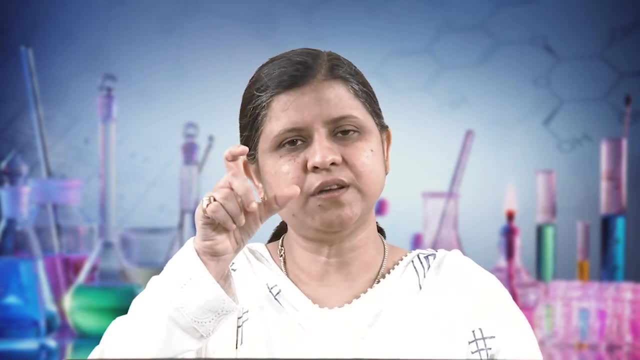 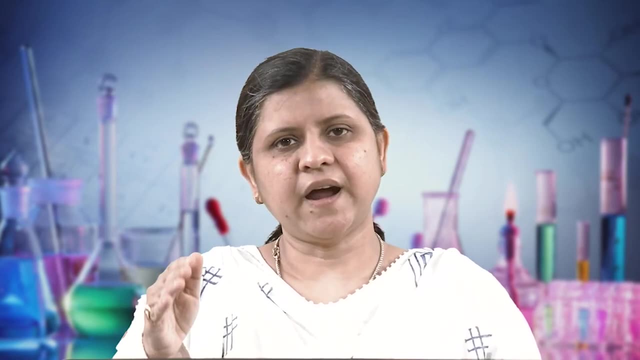 like in one plate, only cornered. Okay, So this is the limitation: The corners which is free for hot fluid. that will remain open, otherwise it will be closed. and on second plate we have to open the space for hot fluid to move. okay. 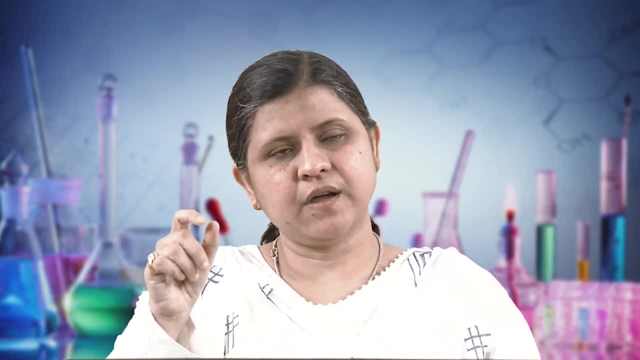 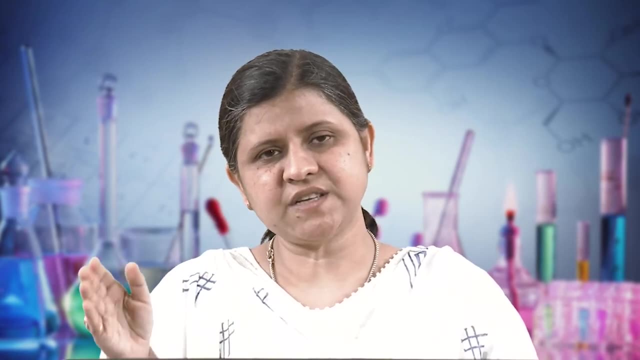 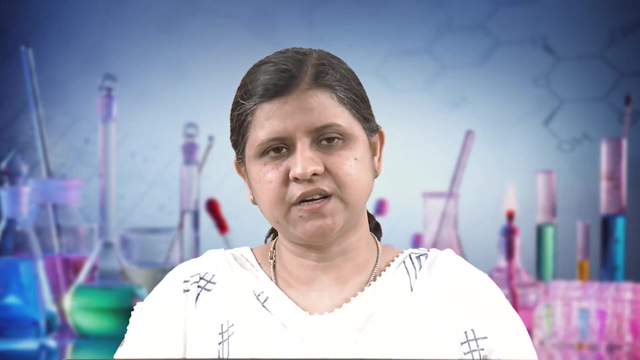 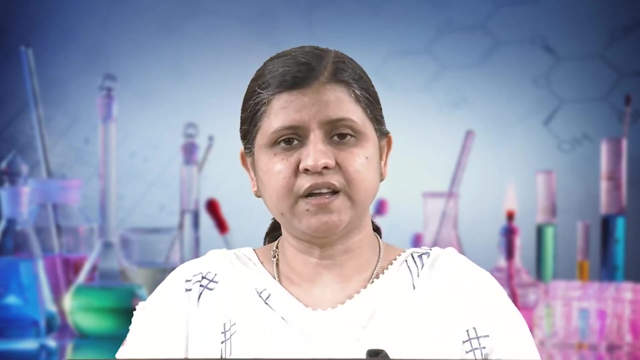 So, accordingly, we can place the. so, accordingly, we can weld the corners. okay, So as far as welding, gasketing or bracing is concerned, the structure over the plate will remain same, as we have already discussed. okay, So welding is done when we are dealing with high corrosive fluid, when we are dealing 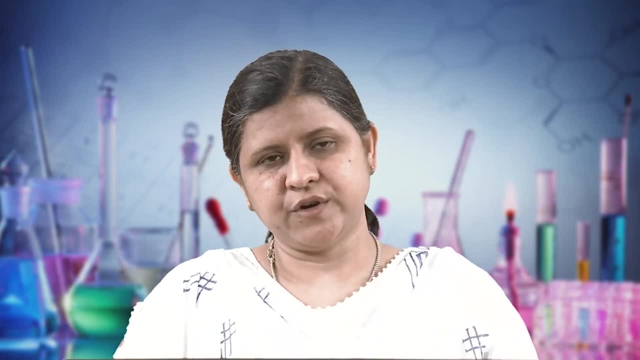 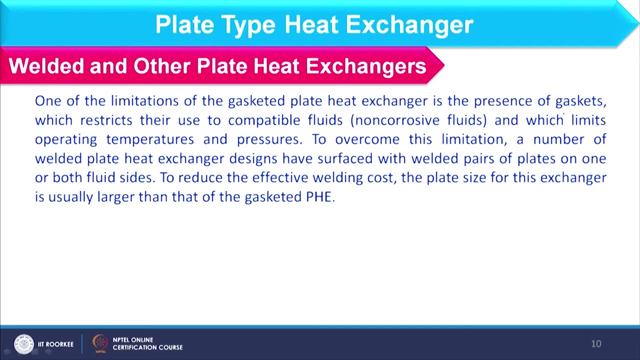 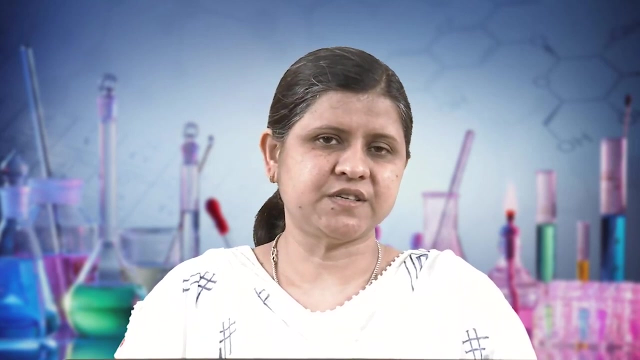 with high temperature and high pressure of the fluid? okay. Again, we have the disadvantage with welded plate because it is permanently joined. okay, So that will be difficult for cleaning purpose. So these are basically advantages and disadvantages, and in which case, which type of plate heat. 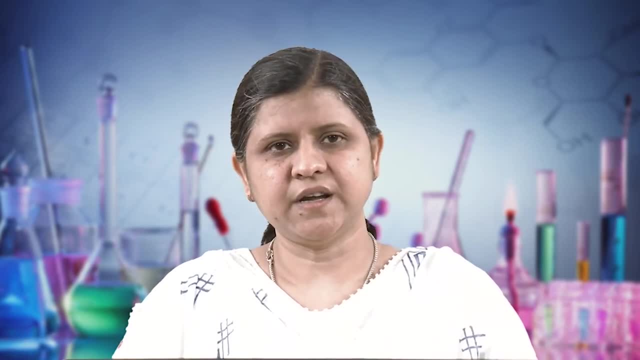 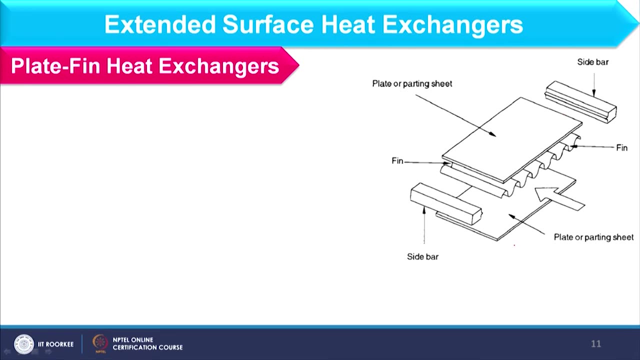 exchanger should be used. all these we have already discussed. Okay, Thank you. Thank you, And now we will focus on extended surface heat exchangers. If you see, here we have the schematic of this. Extended surface means we are basically using the fins. okay, 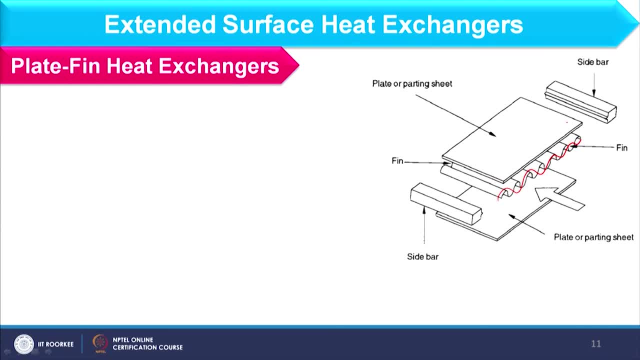 And these fins are basically placed between two plates. okay, If you see, these two plates are there and fins are in between, and here at the side we have side bar. okay, So inside this fin we have one fluid. another fluid would be over the plate, okay. 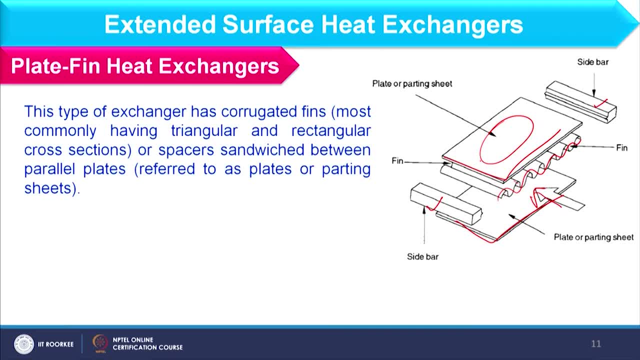 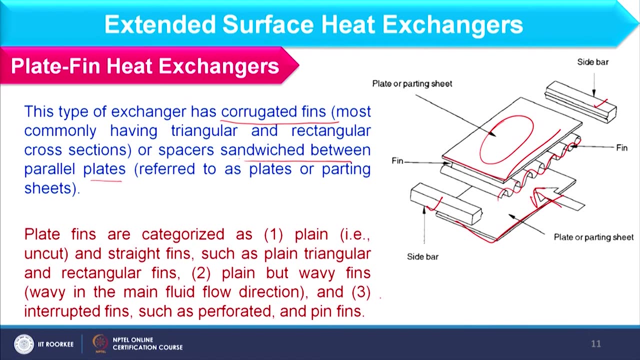 So this is basically plate fin heat exchanger. So this type of exchangers has corrugated fins or spacers which are sandwiched between parallel plates, as we have just discussed. okay, and plate fins are categorized as plain and straight fins, Okay. 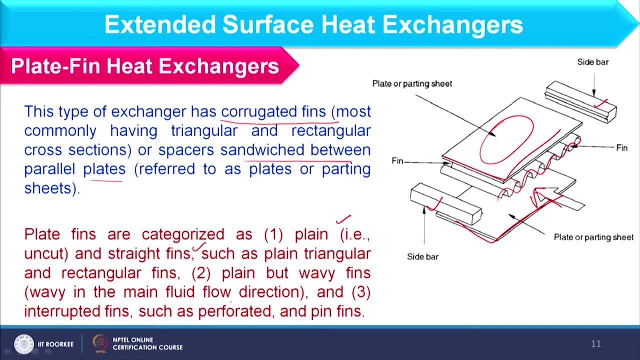 as plain triangular and rectangular fins, like we have this type of fins or we have this type of fins, okay, So this is rectangular and triangular type of fins and in some cases it is wavy fins, as we are discussing, as we can see here. okay, and interrupted fins with. 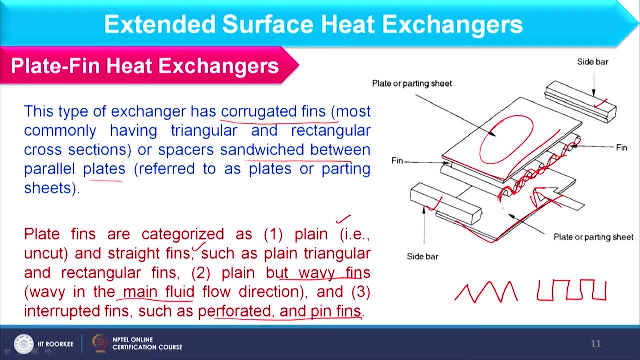 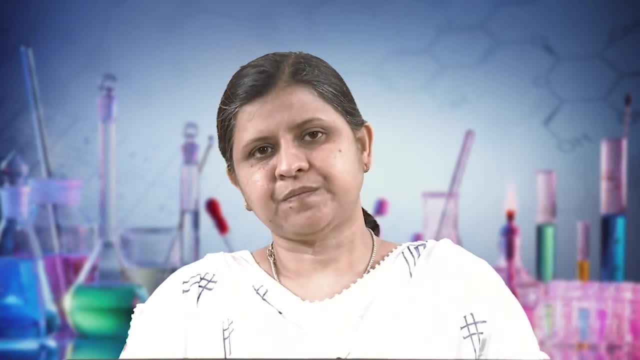 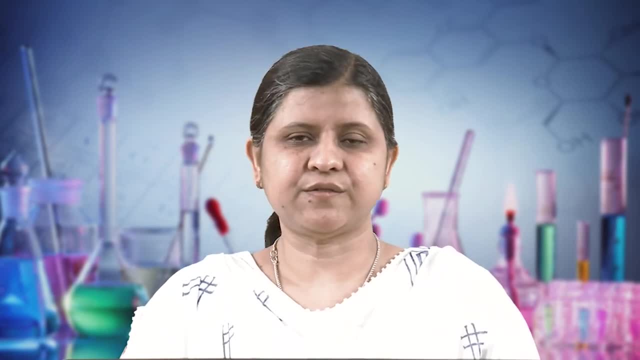 some perforation and pin fins, okay. So because of this perforation or pin fins, we can have more turbulence, so we can increase the heat transfer coefficient, okay. Now the point is where I am using this fins okay and what I am saying, that extended surface. 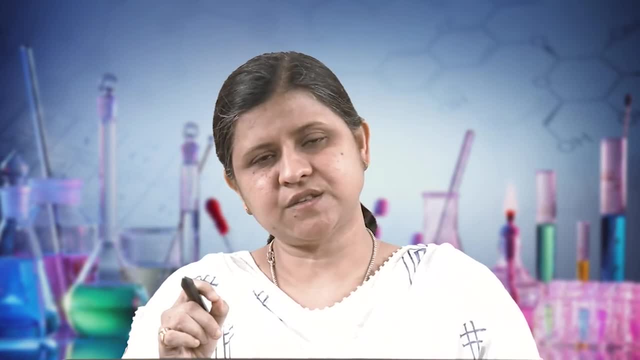 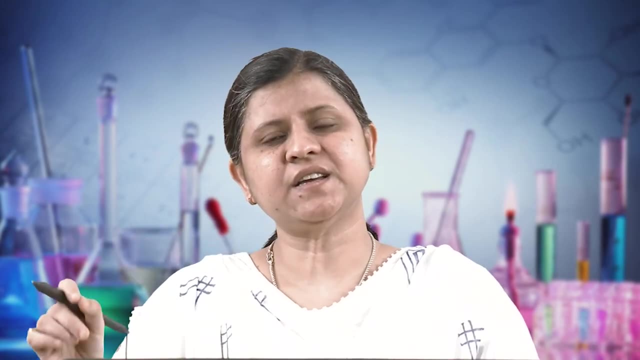 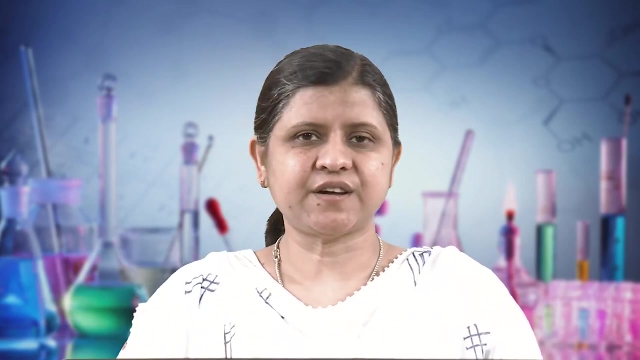 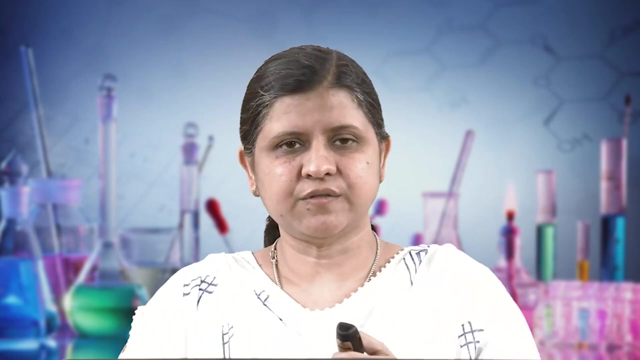 where I am finding lesser heat transfer coefficient. there we are considering plate fins because we are increasing the heat transfer area in the surface In that particular section. okay, So it is called the extended surface because we are extending the heat transfer area in a particular region. okay, So because of that, we are using 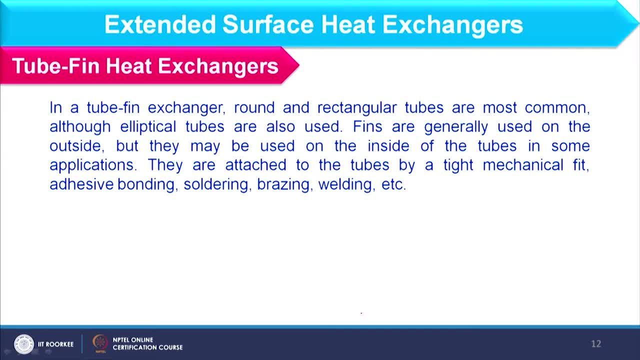 plate fin heat exchanger and tube fin heat exchangers we also use and these type of heat exchangers are round and rectangular tubes are most commonly round and rectangular tubes are most common And sometimes we also use elliptical tubes. okay, and fins are generally used on the outside. 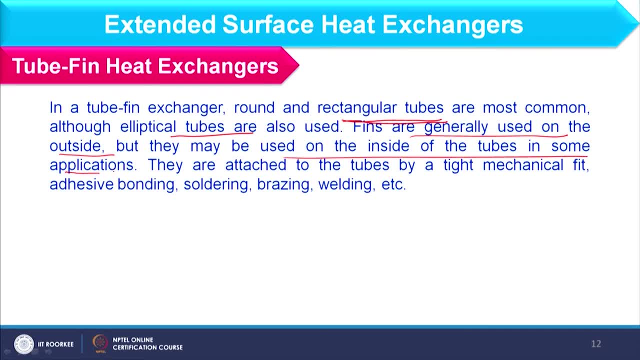 however, in some cases inside also, we put the fins for some specific applications And these fins are attached to the tubes by tight mechanical fit, adhesive, binding, soldering, brazing or welding in this. So in this way we can consider, We can place the fins in the tubes. Now, if we focus on this schematic, here we have the 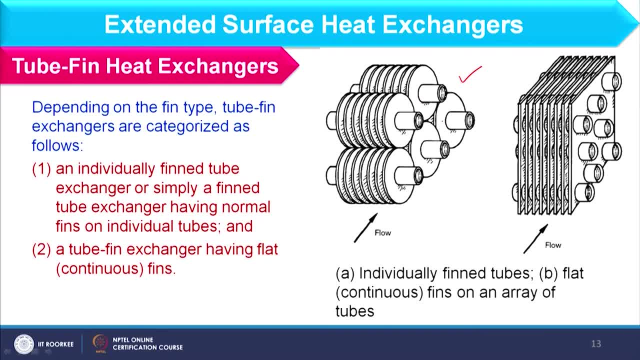 tube fins. okay, and each, if I consider this image here, we have this tube. inside this tube, fluid will move and over this tube we have this disc type of fins. okay, And because of this disc type of fins, the shape of this fins is tube type. that is why. 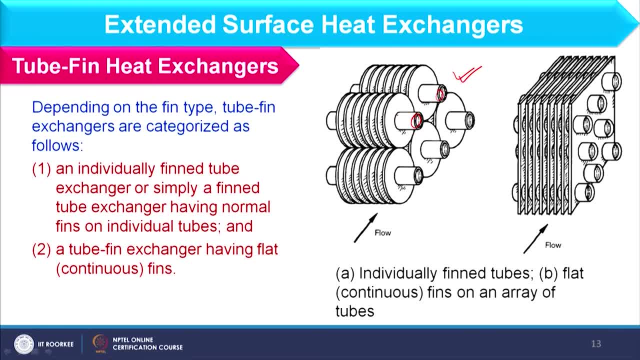 it is called as the tube fin and it is attached over the tube. okay, So it is like when you put the cds in a tube, side by side. so it is this type of a structure and this we call as individually finned tubes. And secondly, we have number of tubes and we have array. 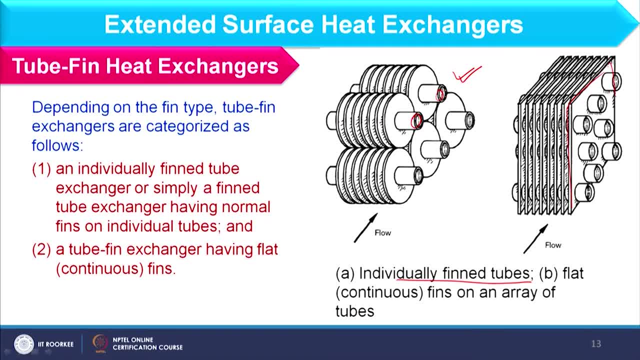 of fins. okay, This is basically array of fins and this we called as flat fins- on an array of tubes, tubes, okay, So in this way, this is, the tubes are arranged in a definite pattern. So this is basically the array and we are considering the plate fins over here. but because it is 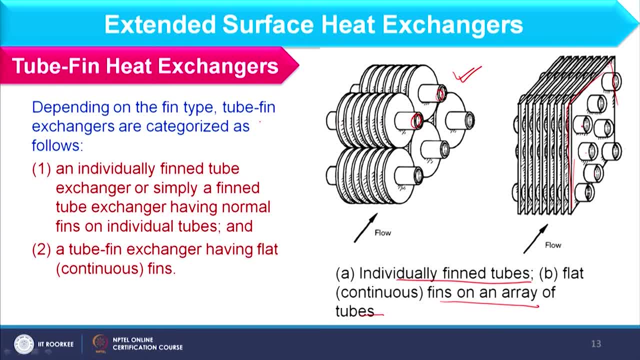 inserting over the tube. it is called tube fins. So, depending on fin type, fin tube exchangers are categorized. So, depending on the fin types, tube fin exchangers are categorized as individually: fin tubes and tube fin exchangers having plate fins. okay, as we have just discussed. okay, 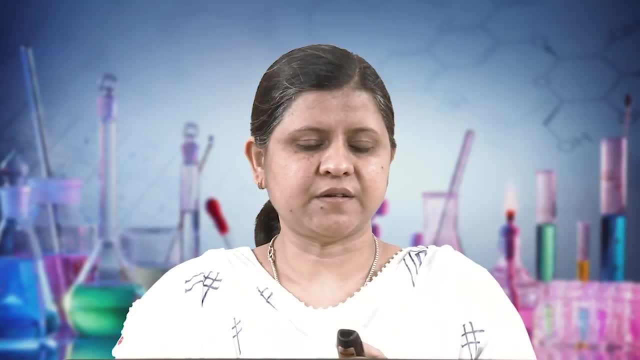 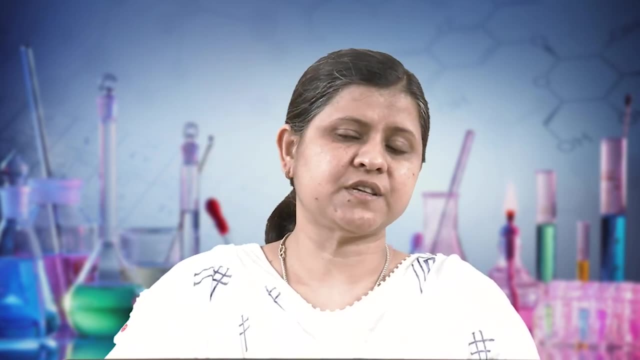 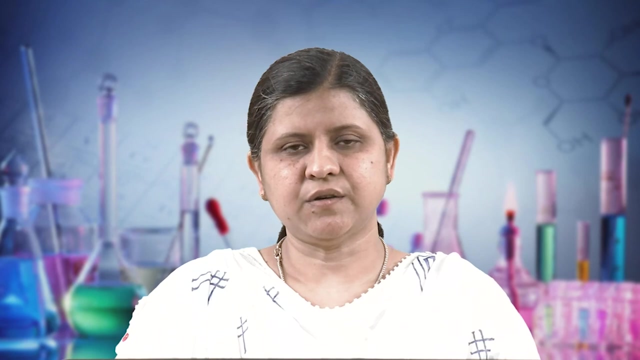 Now we are focusing on direct contact heat exchangers. So direct contact heat exchanger- we have already discussed when I am not having a separating wall between 2 fluids, So hot and cold fluids will come in direct contact with each other, okay, So what will happen? 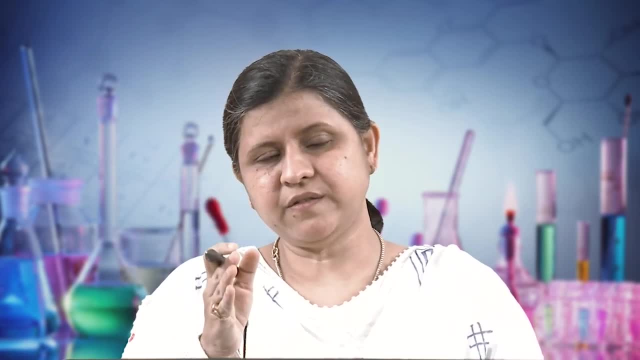 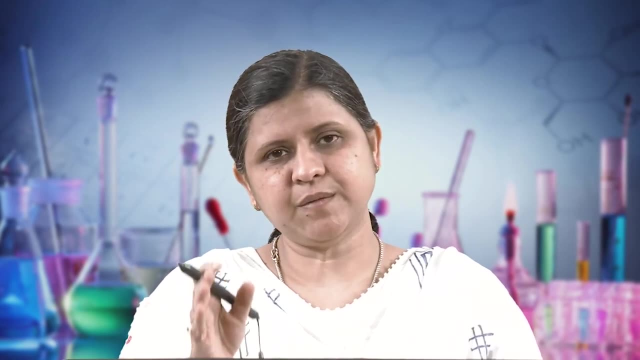 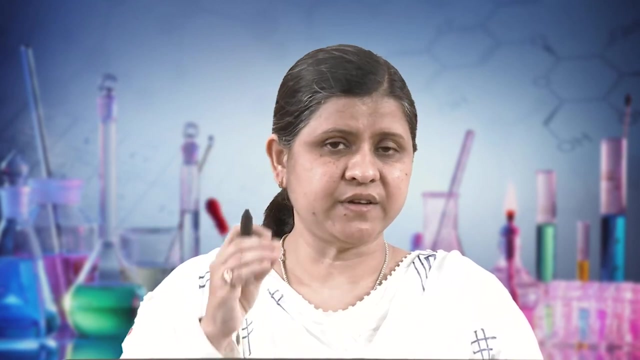 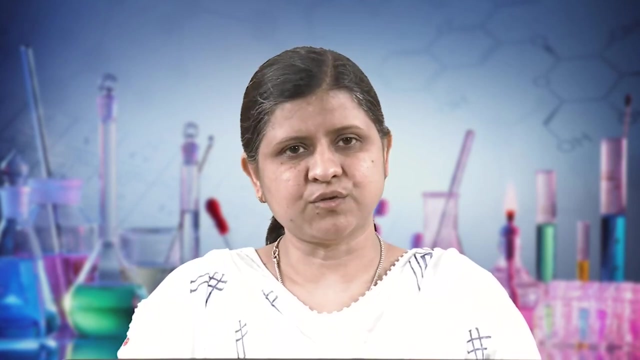 if I am considering the separating wall, will provide the resistance to flow the heat okay And in direct contact type that separating wall is not available. heat can be transferred from one fluid to another fluid directly without any resistance. So in that case we find high rate of heat transfer okay and that is obvious. 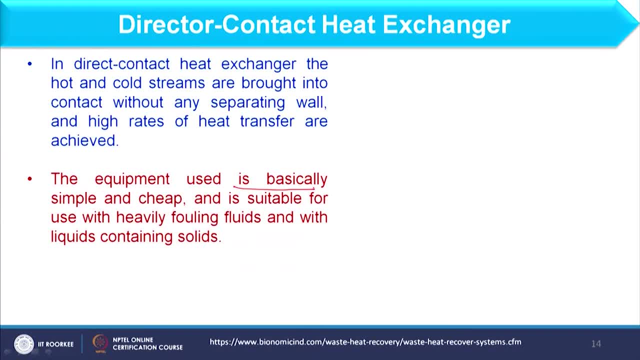 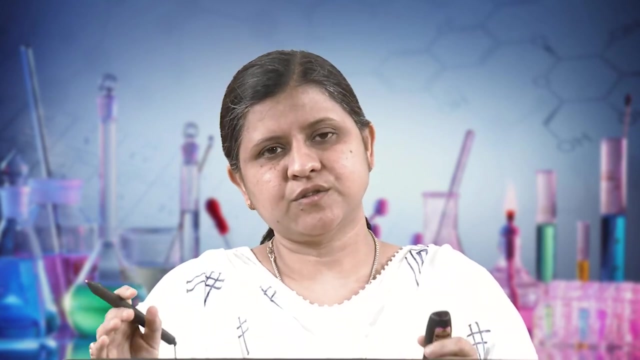 also. So the equipment used for direct contact type is basically simple and cheap, and it is suitable for use with heavily fouling fluid and with liquid containing solids. okay, So when I am dealing with high fouling fluid where we can have reduced heat transfer coefficient, 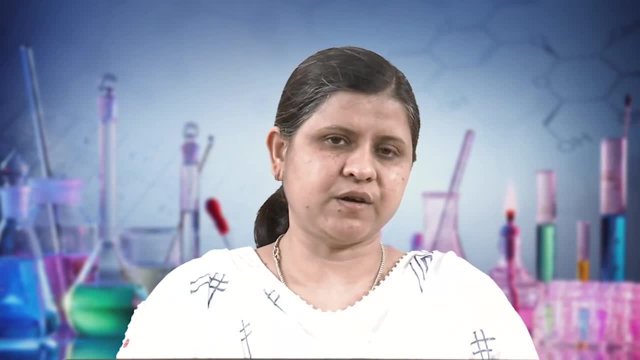 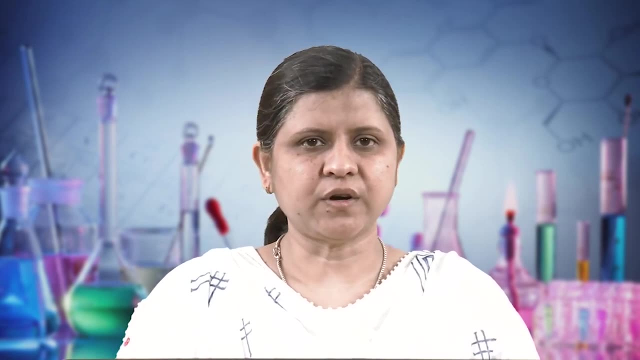 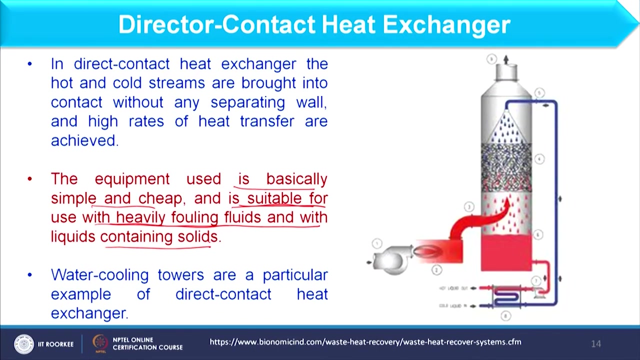 so that fluid can be handled easily in direct contact type. okay, because further resistance is not offered in heat transfer. okay, So water cooling tower, Water cooling tower, So air coolers are example of direct contact heat exchangers and this is the one image. 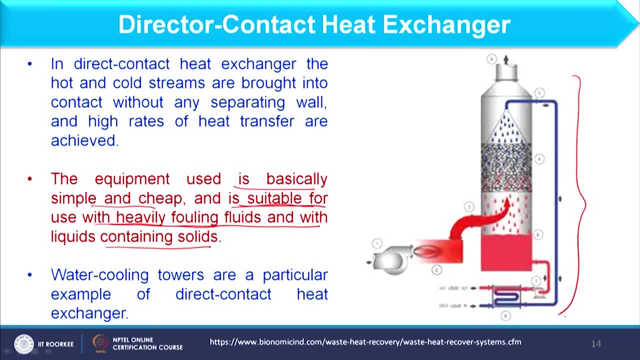 above and here I am having one image of direct contact heat exchanger and details you can find here. So here hot air, hot gas, enters into this and it exchanges heat with the cold water which is coming from the top, or cold liquid, And then subsequently cold liquid is heated up and hot gas is cooled down and exits from. 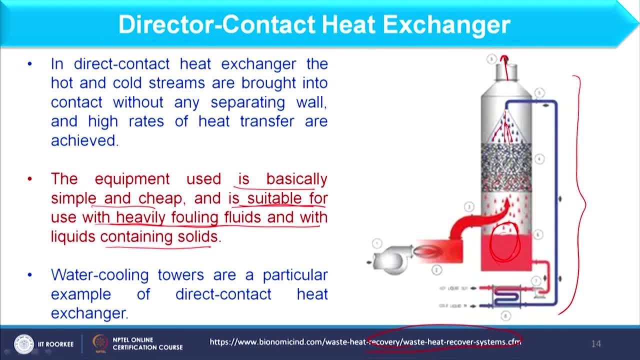 the top And this hot fluid, hot liquid further gets cooled in this heat exchanger where heat transfer occurs. between this, where heat transfer occurs from this fluid, and then it cools down and further recycles back to the top. So this is the one image of direct contact heat exchanger And here I am having one image. 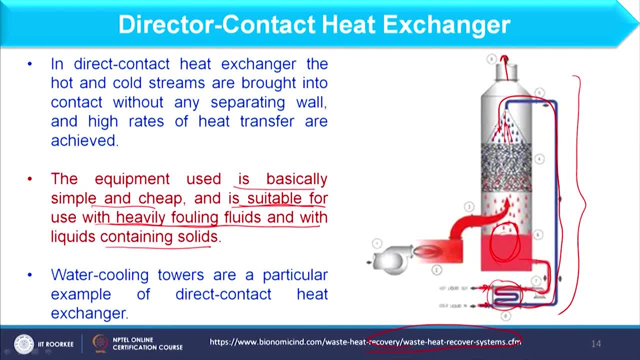 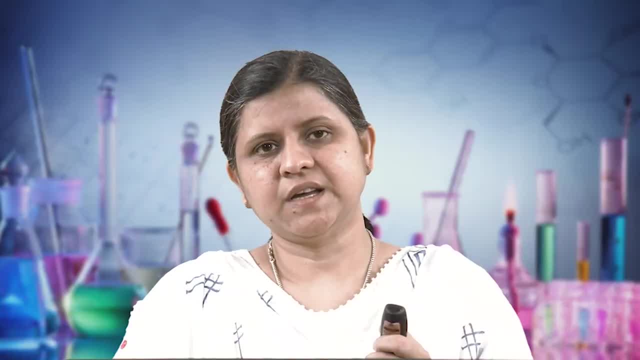 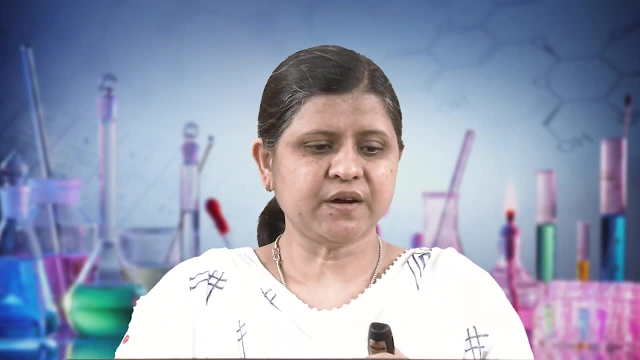 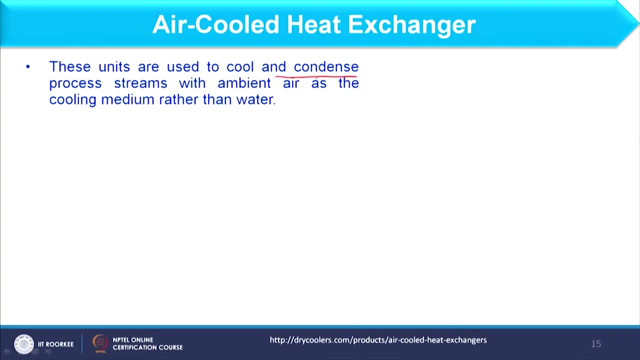 of cooling tower. okay, and this is basically the assembly of cooling tower we usually use to produce cold water in chemical plant. okay, So that is about the direct contact heat transfer. Now I am having air cooled heat exchanger. okay, Air cooled heat exchanger, air cooled heat exchanger are used to cool and condense process. 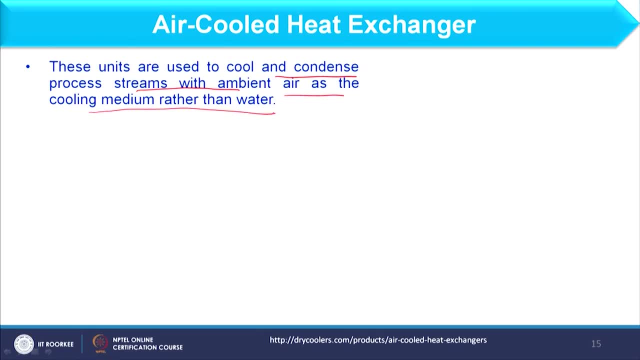 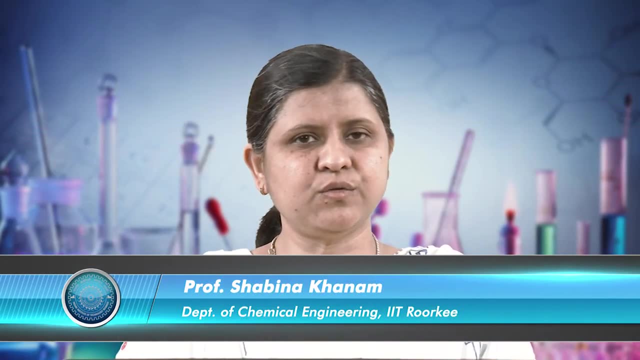 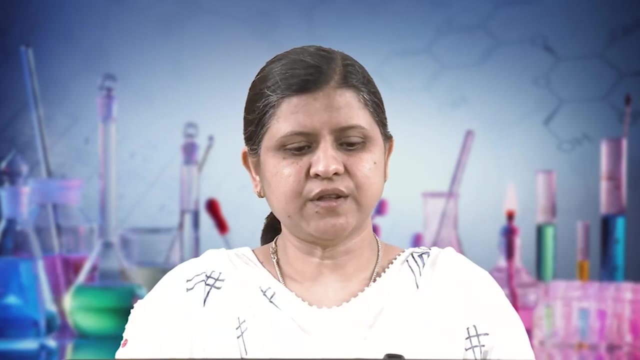 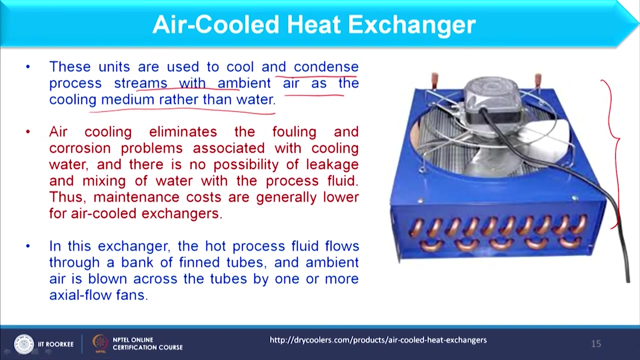 stream with ambient air as cooling media rather than water. So usually for condensation purpose we use water, okay, but here we are using air as a cooling media. and second fluid will definitely be the vapor which is to be condensed. okay, So when the fluid? so, if you see this schematic, when the fluid is to be condensed, that fluid. 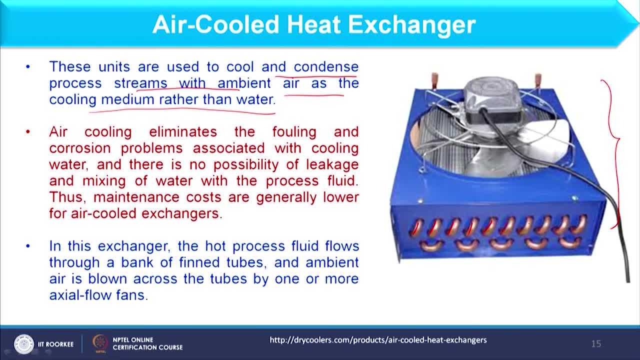 should move or should flow inside this copper tubes. okay, inside these copper tubes and this fan we are using, And this fan we are using to throw the air over these tubes and therefore this vapor which is flowing in the copper tube can be condensed and vapor hot and hot air can be. 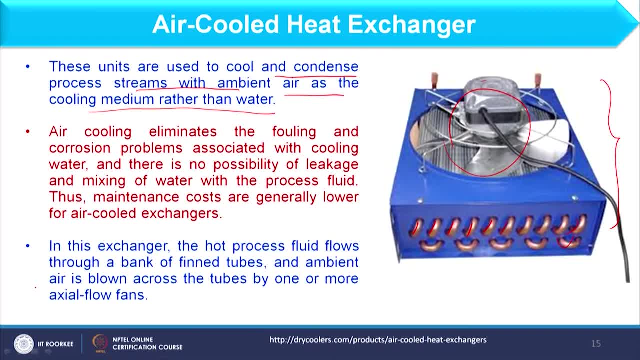 exits from the bottom. okay, So in this air cooled heat exchanger, if I am putting the fan at the top, okay, Okay, Top means before the process is going on. okay, because once air will be thrown by this fan, then condensation will take place. 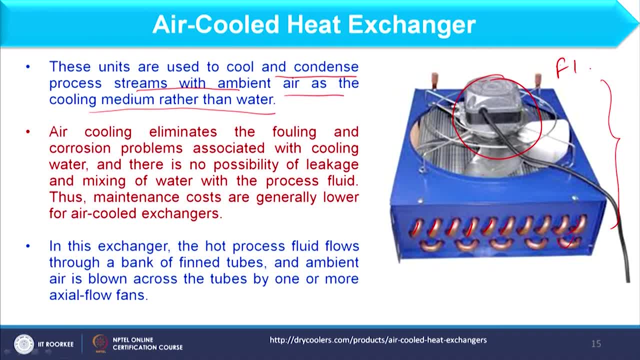 So this type of placement of fan we called as FD fan or forced draft fan, because it forces the air in the system. It means it create positive pressure in the system. okay, On the other hand, we can place fan at this side also instead of top side. 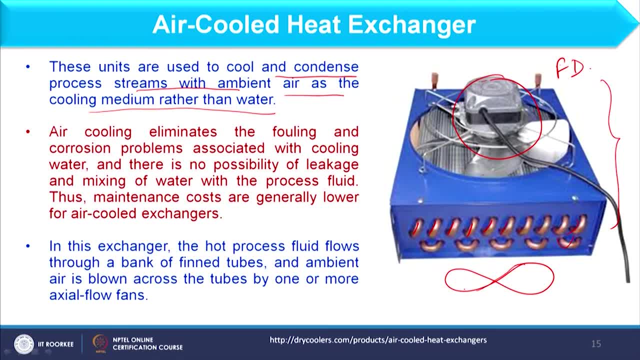 Okay, Thank you. So, considering this, it means it is basically sucks the air. okay, It basically sucks the air, and it basically sucks the air as it is placed after the operation. okay, So this type of fan is called as ID fan or induced draft fan. 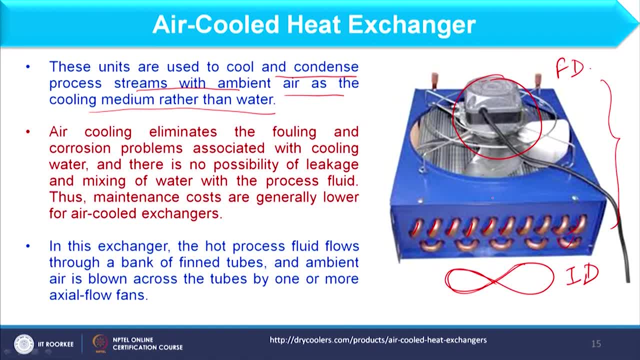 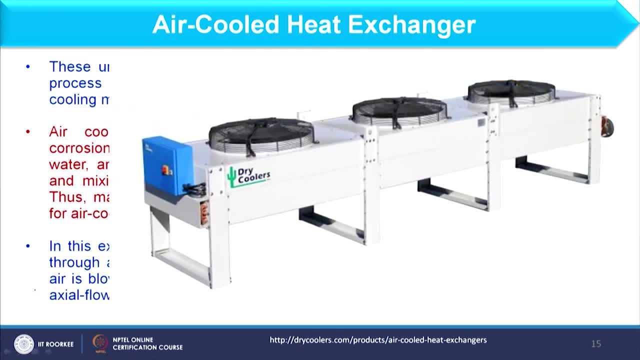 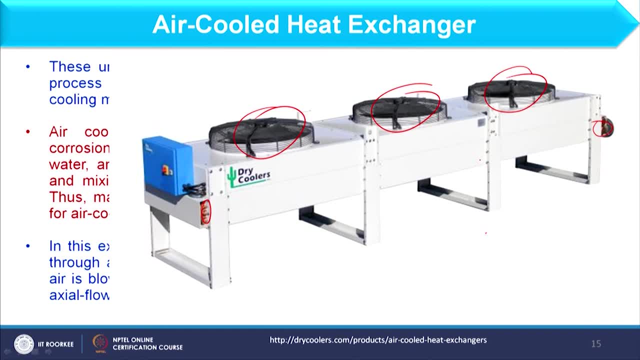 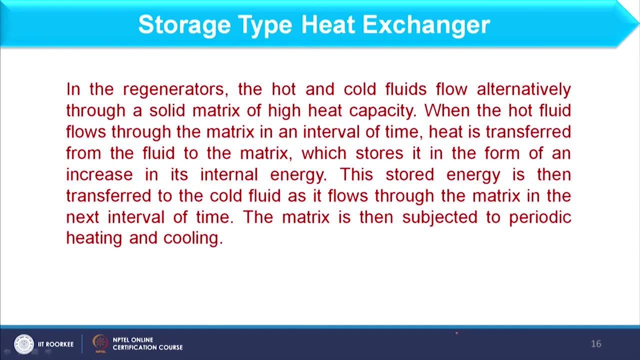 we have the copper coiling inside this, So this is another example of air cooled heat exchangers. You can find details in this site And now we will focus on storage type heat exchangers. Okay, And storage type heat exchanger. these are basically called as regenerators, where hot. 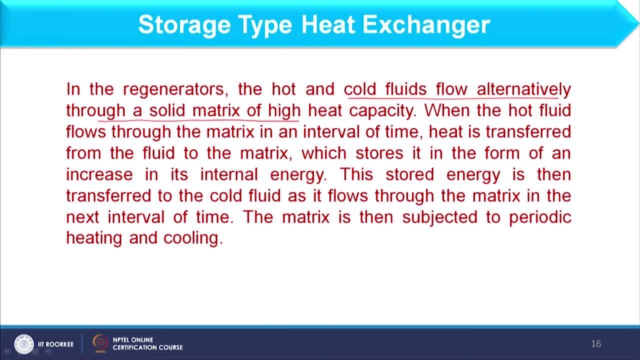 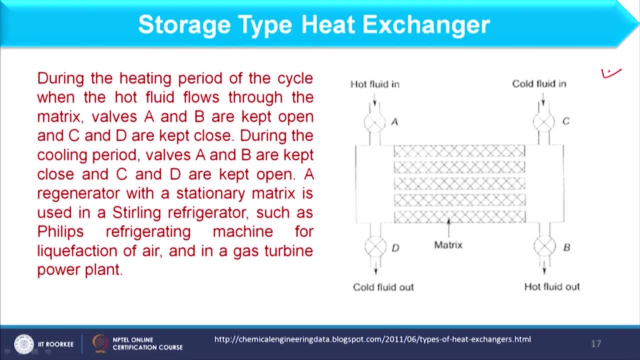 and cold fluids flow alternatively through a solid matrix of high heat capacity. Okay, To illustrate that, let me focus on this image Here. if you see, in this heat exchanger we have the solid matrix. Okay, This is the matrix. zigzag formation is there? 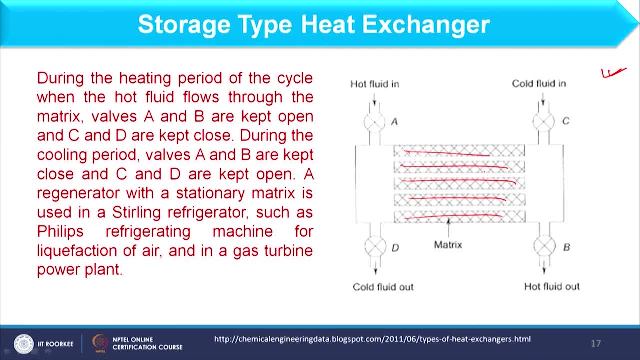 So this is the solid structure. Or we can consider that as packing, And hot fluid enters at, and hot fluid enters from point A and exits from point B, Cold fluid enters at C and exits at D. nozzle, Now what will happen Now in this storage type heat exchanger, hot fluid first moves and at that time cold fluid. 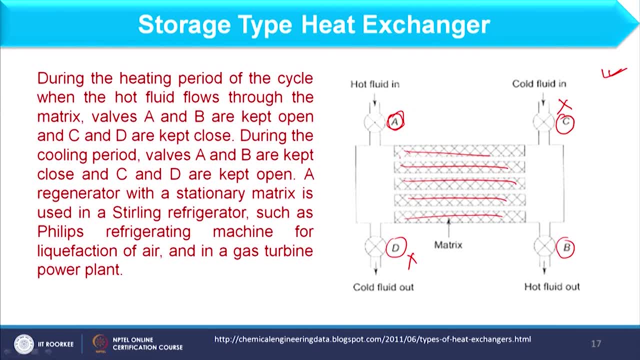 nozzle will be closed. Okay, So hot fluid, whatever is moving, It will enter into this, transfer its heat to this matrix and then exits from here. Okay, Second time, what will happen? This will be open and this will be closed, Okay. 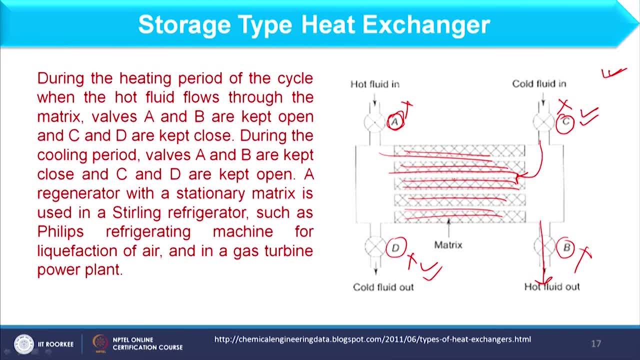 So cold fluid will further pass through this and then it will take heat from the matrix and then exits from here In this way. this is basically storage type heat exchangers And here this matrix is moving. It will enter into this, transfer its heat to this matrix and then exits from here. 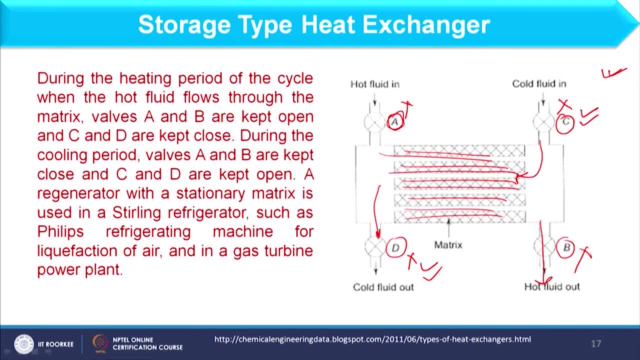 So here this matrix is used as a media to store the heat And these are used in sterling refrigerator such as Philips refrigerating machine for liquefaction of air, and in gas turbine power plant. So these are some of the application for storage type heat exchangers. 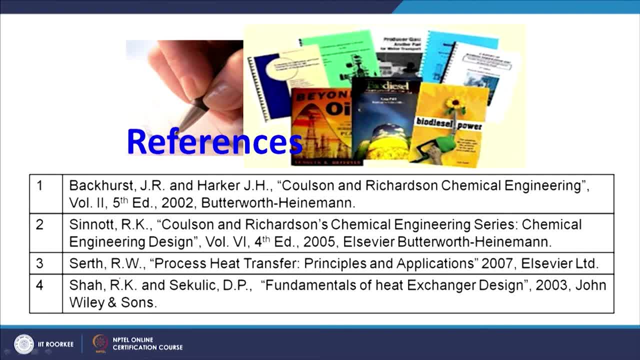 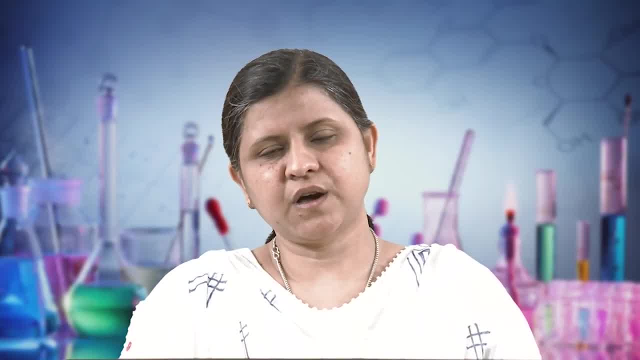 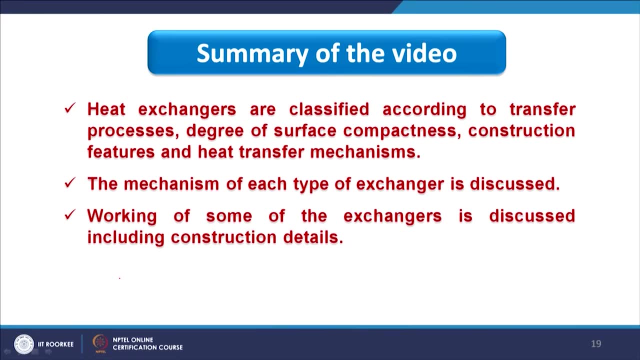 And here the references are there, which you can use to study this topic more clearly and in more detail. Now let me summarize this video. Now, as far as this summary is concerned, this is the summary of lecture 2 and lecture 3 of week 1, okay, where we have discussed the classification of heat exchangers. 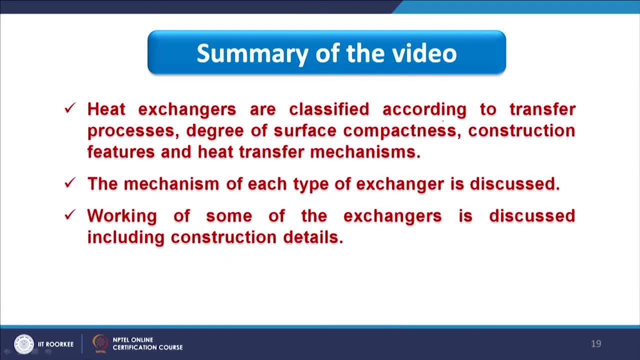 So summary goes: as heat exchangers are classified according to transfer processes, degree of surface compactness, construction features and heat transfer mechanisms, Mechanism of each type of heat exchanger is discussed in detail. And what is the heat transfer mechanism? Okay,